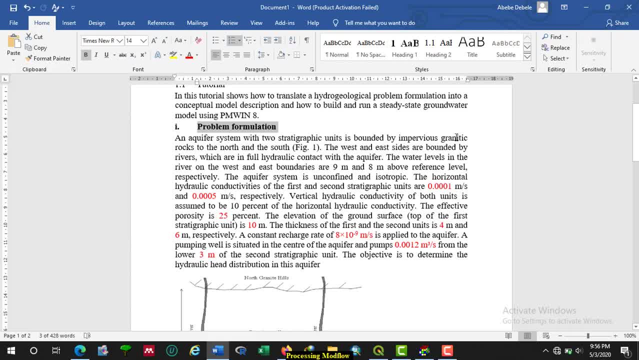 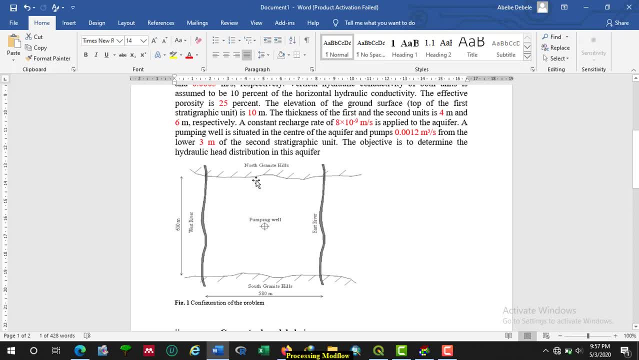 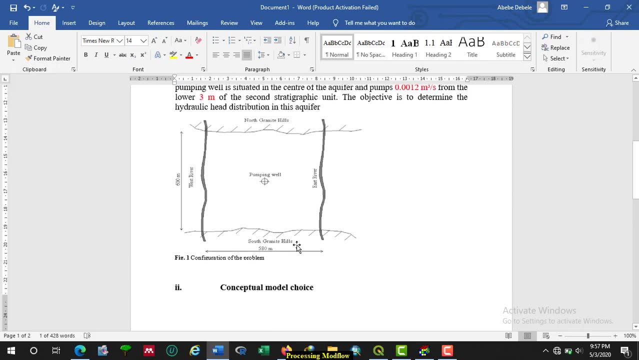 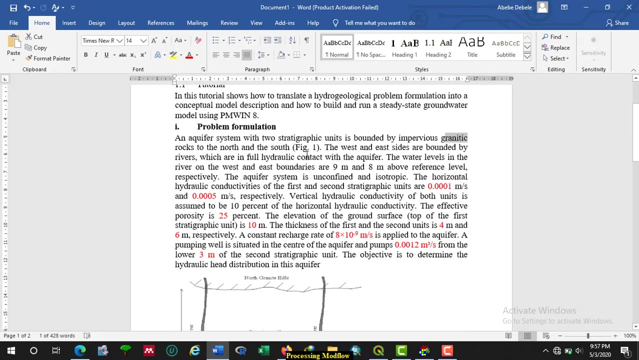 impermeable geological formation which is a granite to the north and south and you can see here on the figure: the north boundary is granite geological formation and also the south boundary is granite geological formation. both geological formation are impermeable geological formation. 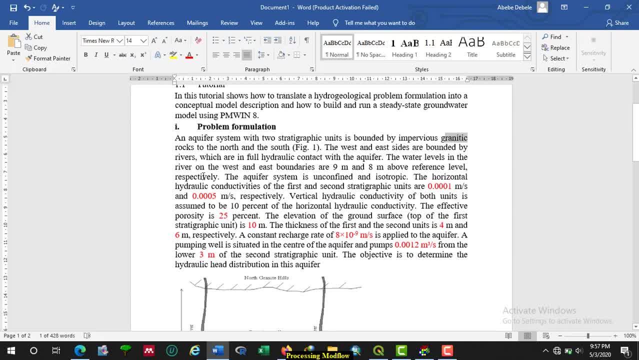 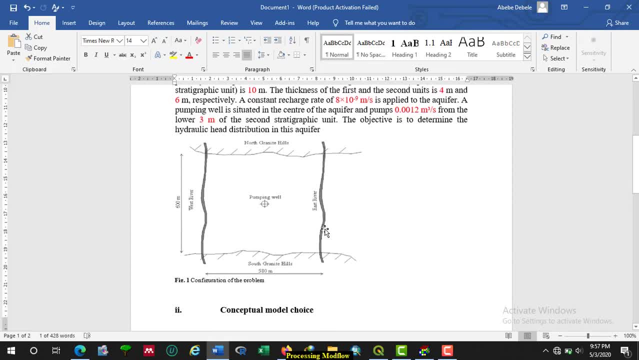 The west and east side are bounded by river, which are full geological formation. Also, the left and west boundary are bounded by river, which appear to be generally highly contact with the aquifer. Here the west boundary is river and also the west boundary is river and this river. 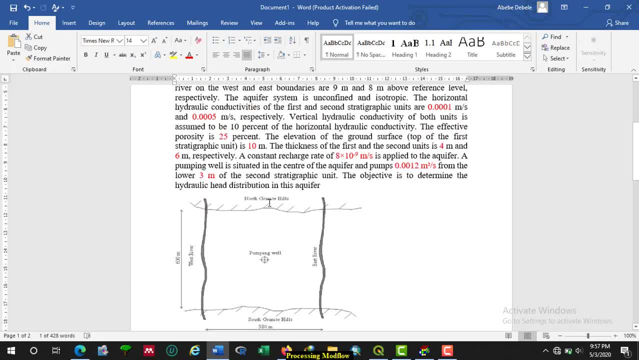 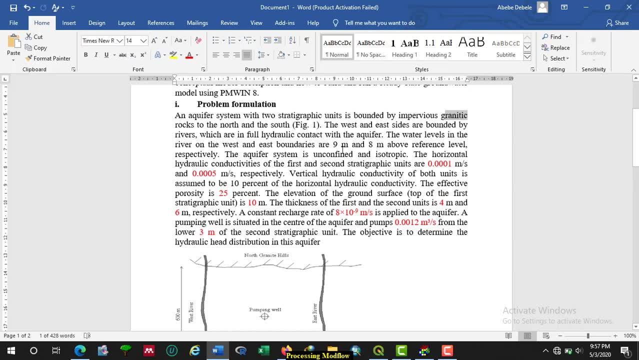 is fully highly contact with the aquifer. The water level in the river on the west and east boundary are 9.0 m and 8.0 m above the reference level. So here the water level at theénwert level is 9.0 m. Here the nゲureías are verdadeísTake nước d میробândềinsägnwczásàä was by abuse or potentialÕ workforce. æfÉiår выбatændä. æf käyr rounded by eiþbased. 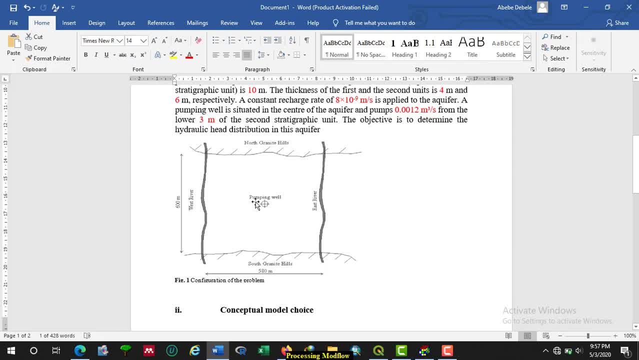 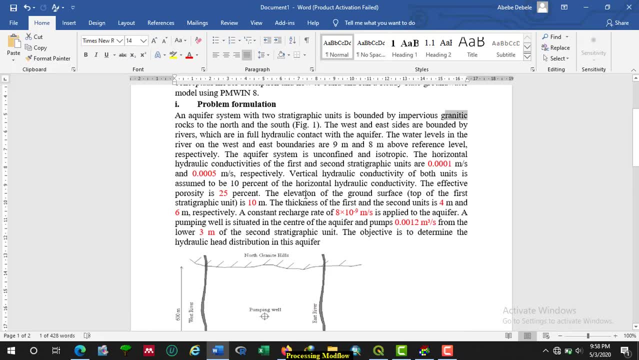 the water level in this river is nine meter and the water level in the east boundary is eight meter. the aquifer system is unconfined aquifer and also isotropic. you know what mean by unconfined aquifer. unconfined aquifer is aquifer which have no confining layer from. 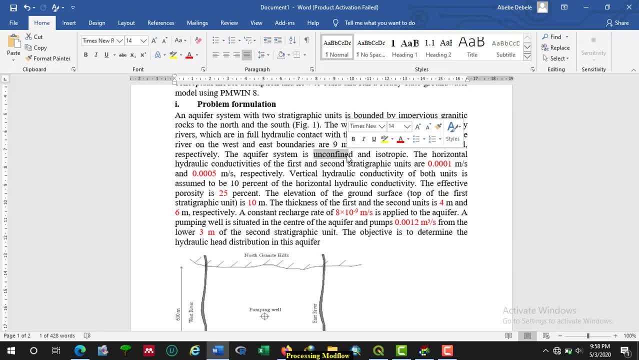 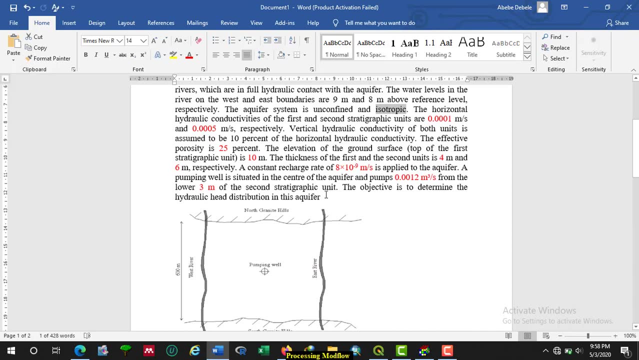 the top and the upper portion of the aquifer is water level and it is isotropic. that means hydraulic property of the aquifer. hydraulic property of the aquifer is isotropic. the horizontal hydraulic conductivity of the first and seventh stratigraphic unit is given for us and the hydroconductivity of first hydrostatic stratigraphic units is: 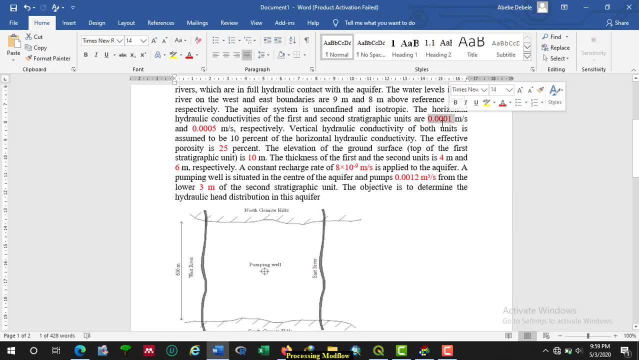 0.001 meter per second and that of the second one is 0.005 meter per second respectively. the vertical hydroconductivity of those units is assumed to be 10 percent of horizontal hydroconductivity. effective density is also given for us, which is 0.25 percent elevation of ground surface, that is, 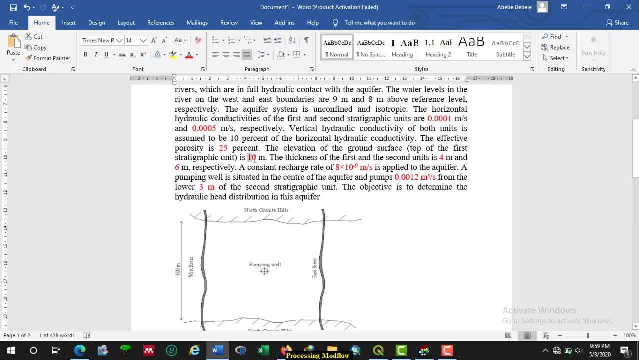 top of the first stratigraphic unit is 10 meter. so the thickness of the strat- the first plus second stratigraphic unit- is 10 meter. the thickness of the first and second unit is given for us, which is 4 meter and 6 meter respectively. the constant recharge rate of 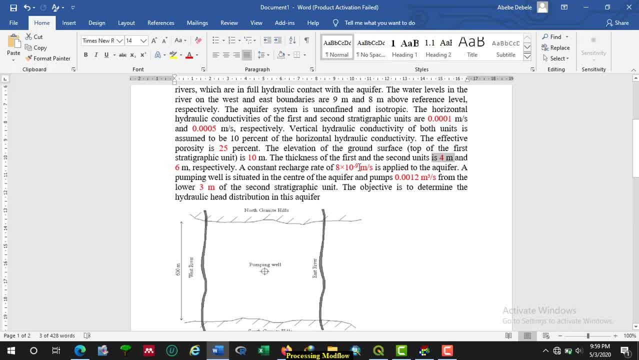 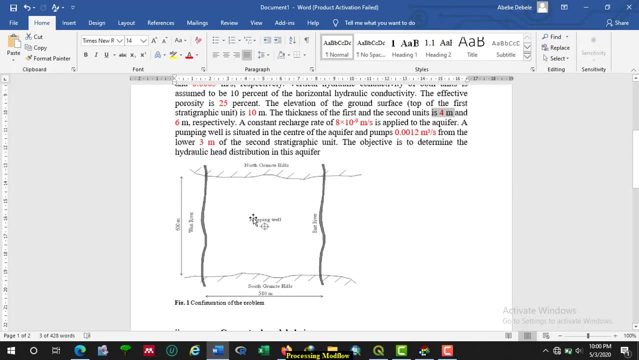 heat times. the rest of minus nanometer per second is applied to the aquifer. pumping well is situated in the centers of the aquifer, so there is a pumping well here and this pumping well is at the center of the aquifer and the pumping rate is this value and from the lower 3 meter of water. second, 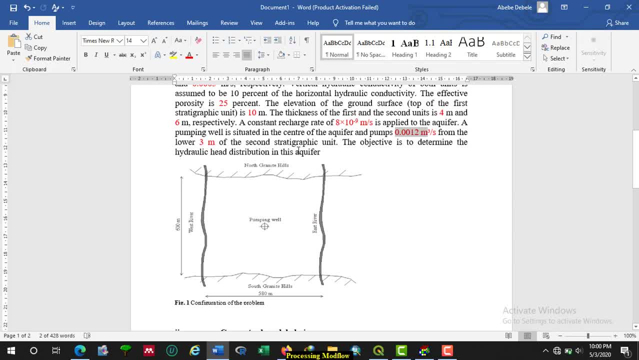 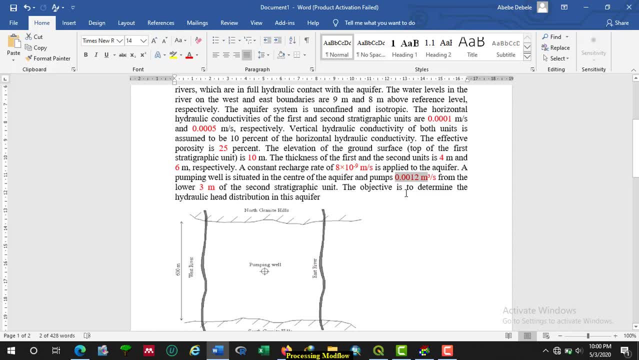 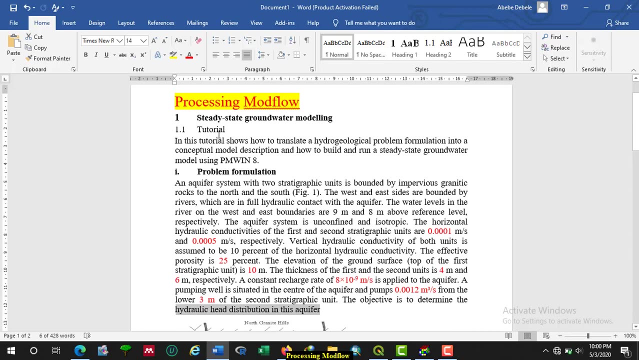 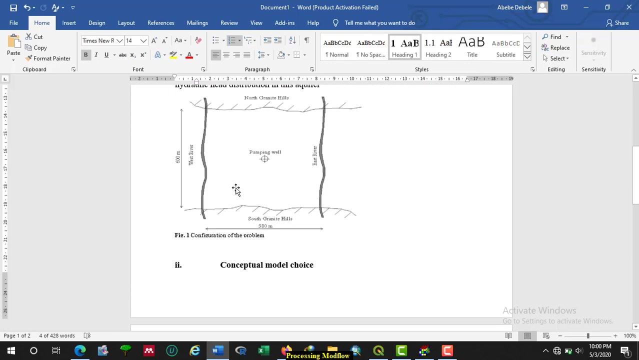 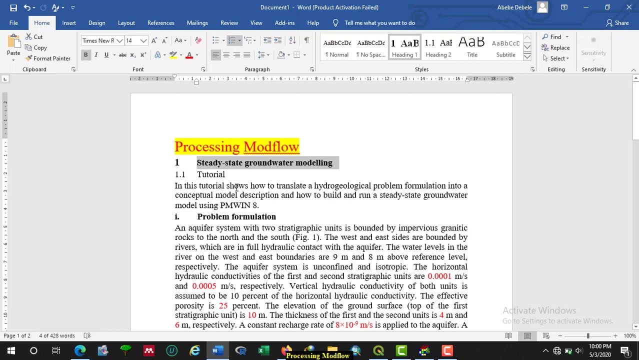 stratigraphic unit here. the main objective of this web lecture is to show you how to determine the hydraulic distribution in the aquifer in the case of a steady-state condition- steady-state ground water flow condition in ground water flow modeling. first we have to have conceptual model. so here we have. 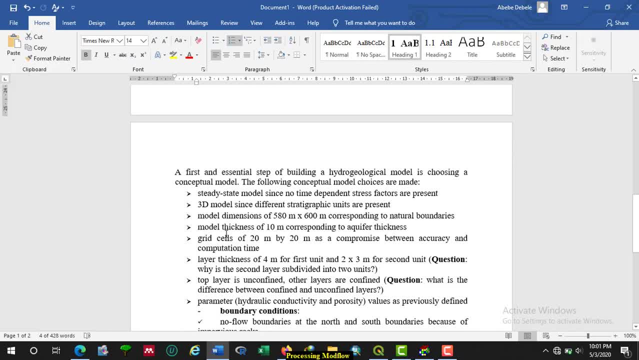 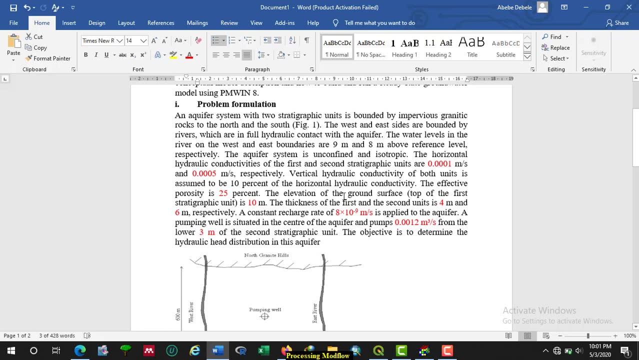 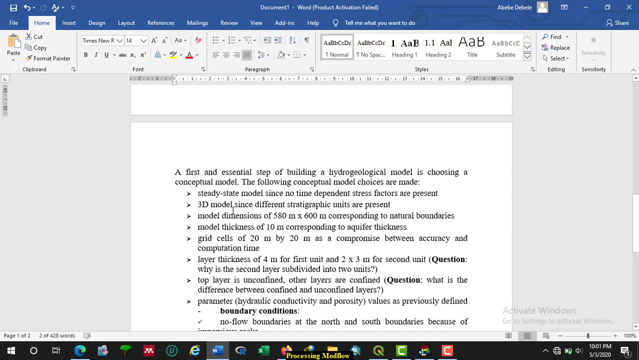 conceptual model choice. the model will be steady-state model, since you know, time-dependent. these factors are presented there. all parameter given for us are not time dependence, including recharge and also pumping rate. all are constant through the time. 3d model, since different stratigraphic units are presented there. 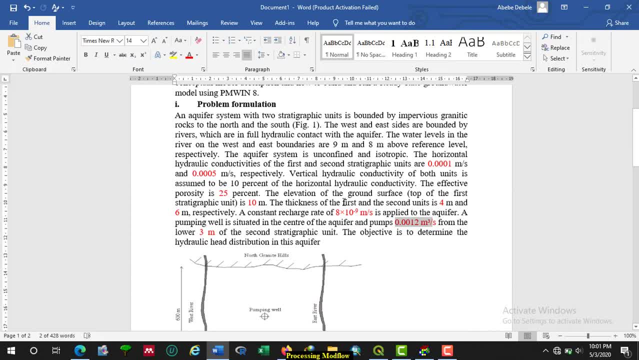 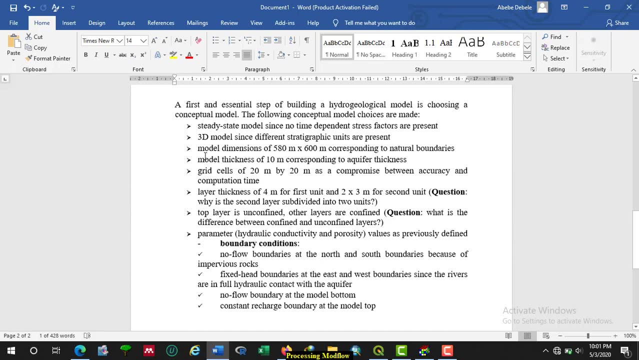 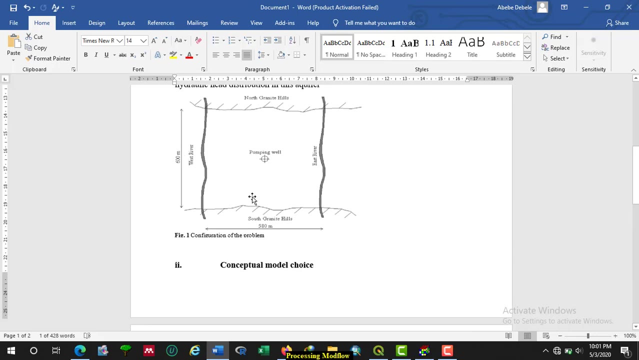 we have two stratigraphic units, stratigraphic one and the stratigraphic two. stratigraphic one having thickness of 6 meter and stratigraphic two having thickness of model dimension is model dimension. you can see model dimension, which is 580 meter by 680 meter. you can see the model thickness on the figure model. 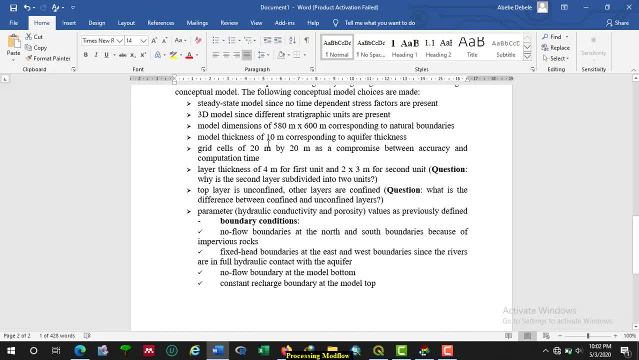 more thicker. thickness: 3 meter by 10 meter, corresponding to the weight of the line of the grid, thicker than the valueari the grid to a vertical. the vertical is 10 meterRIA, whiteboard width barely 0.. rigidity: three meters reach equal, so the model thickness will also be 10 meterける. cash sales will out sync with. 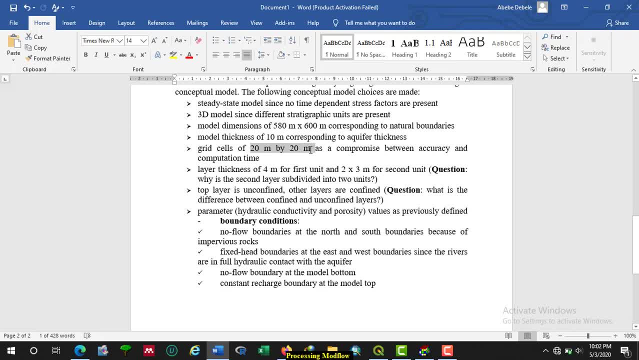 the body size will be reduced. precise distribution of other sit: it is 20 by 20. actually we're selecting the grid sales of the model. we have to compromise. we have to compromise and consistency and condition. Well, this is good either way. when we select small size of grid cell, the accuracy may be good but the 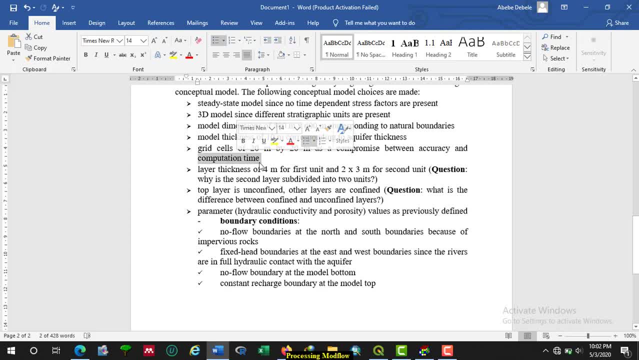 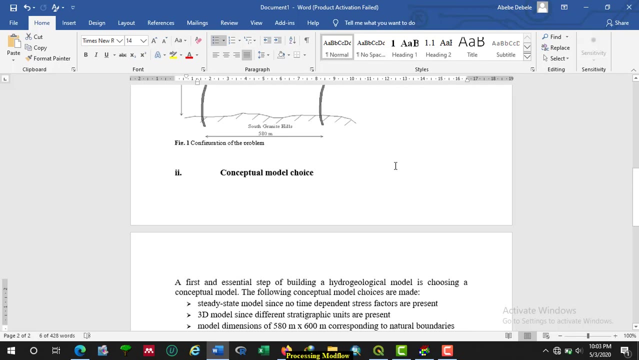 computational time may be long, so we have to compromise both accuracy and computational time. for current, it's better to select this value: 20 meter by 20 meter. layer thickness of 4 meter for the first units and 2 times 3 meter for the second unit. this is because the well pumping well is what 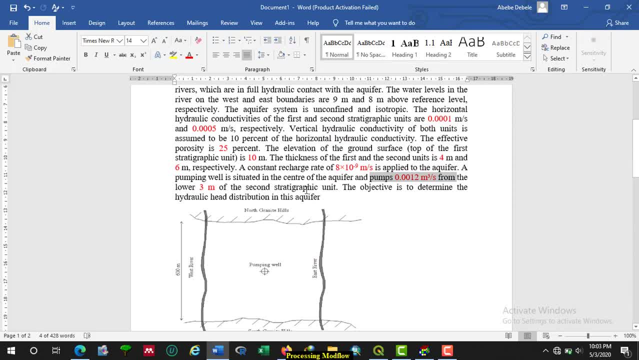 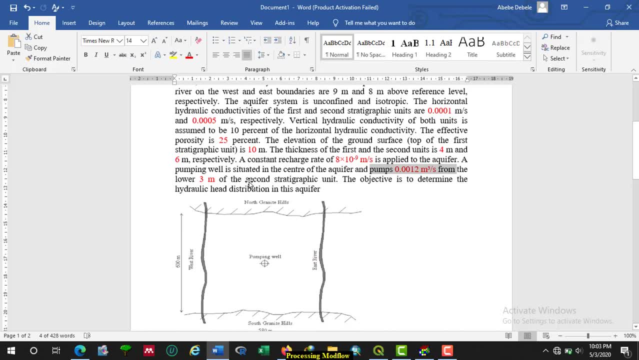 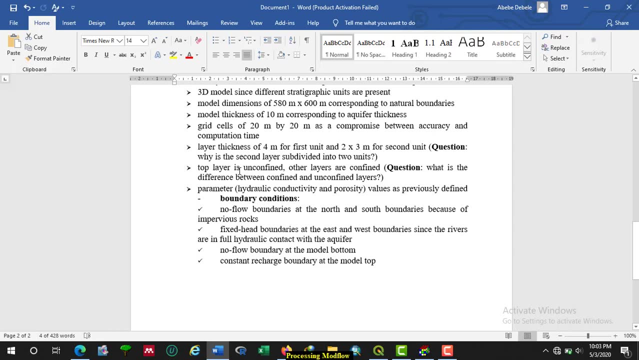 situated at what? the lower 3 meter of the second stratigraphic unit. so we have to divide the second stratigraphic unit into two layer. top layer is unconfined giver and other two layer are what confined givers. you know what is confined giver and what is unconfined giver. 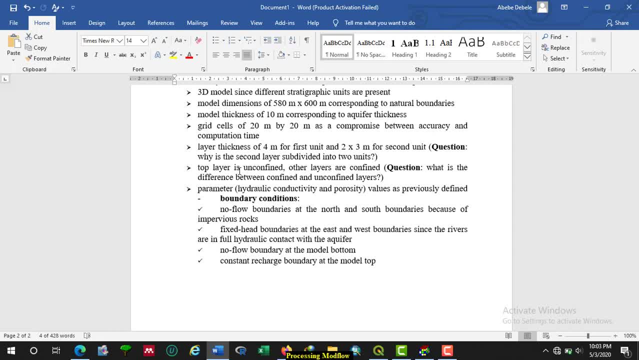 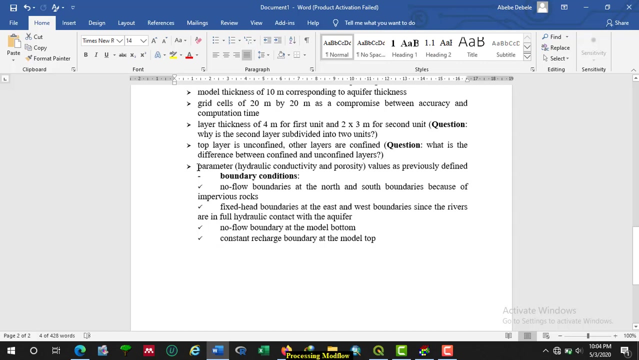 given the case of confined giver, there is some confining layer from the top and layer from the bottom. for unconfined giver the upper, most saturated layer is weather table and there is no confining layer there and here parameter- some parameter are also given for us highly conductive, it is covered. 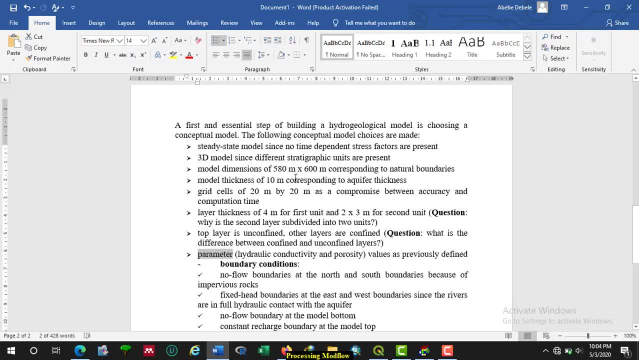 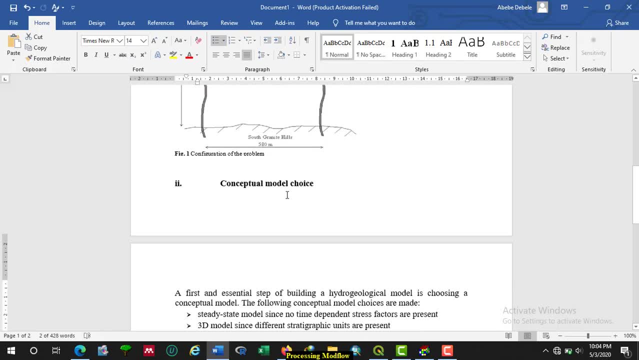 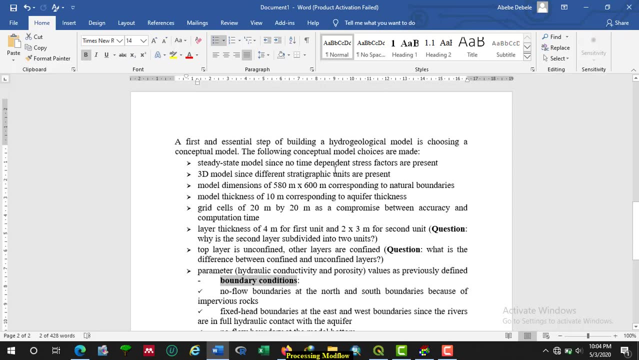 for us, for a statistic for us and you can look at the value of porosity and how do we conducted both vertical and horizontal hydraulic conductivity. boundary condition is also given for us. no flow boundary condition at North and South. you can look as the North boundaries, granite formation and South boundaries also. 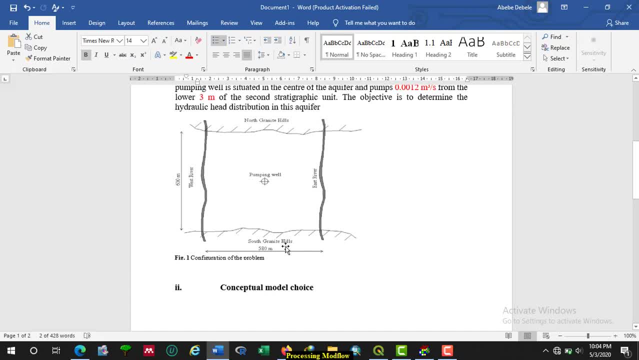 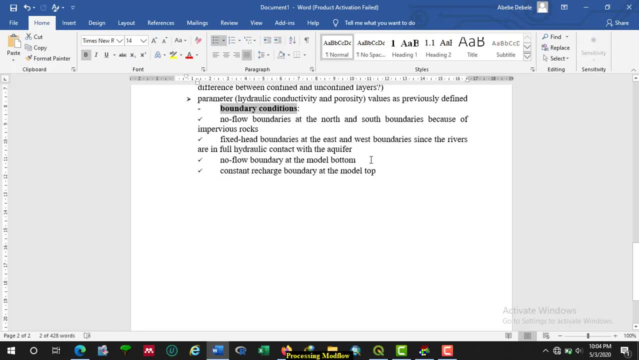 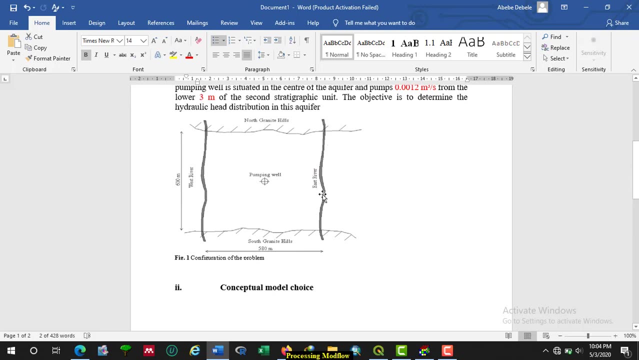 granites formation, granite rock, also impermeable geological formation. fixed boundary at the east and west boundary since the rivers are in full hydrocontact with the aquifer. so this one is fixed head boundary. this one is fixed head boundary. both west and east boundary are what fixed head boundary having. 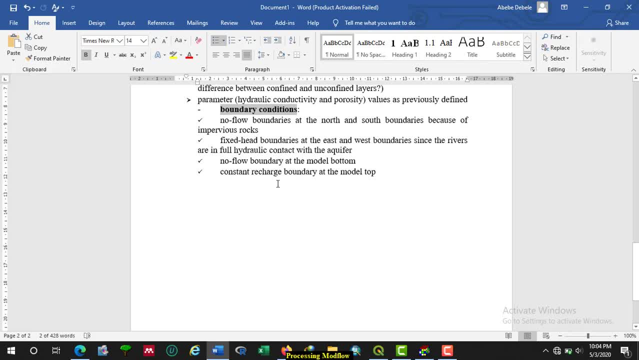 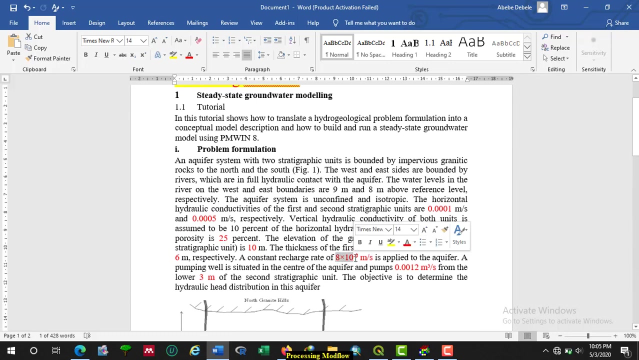 constant head. no flow boundary at the model bottom. that means the bottom of the model is what model is basement of? there is no flow of water from the aquifer to the bottom. constant recharge boundary at the top which is equal to this value, which is equal to a times 10, to the power of minus 9, and we 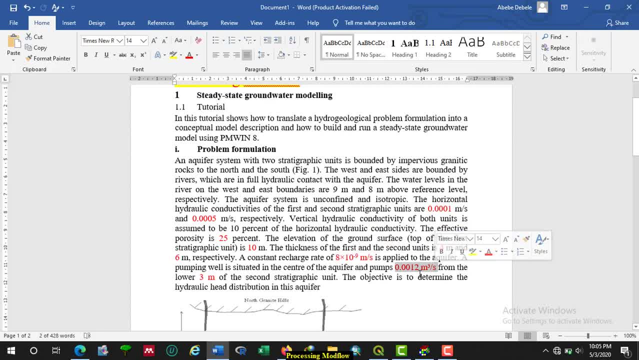 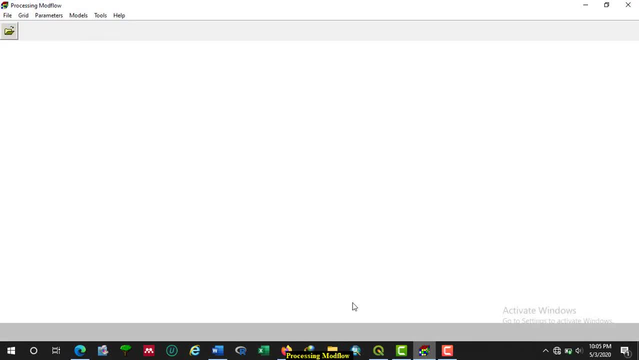 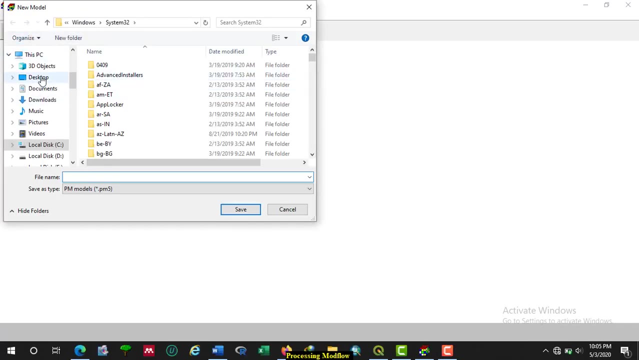 have also bumping or well, boundary of this ready. it starts with modeling. first we have to save our model. to save our model you have to click file, then new model. let us save our model here in dib tutorial and name tutorial. one save once we save our. 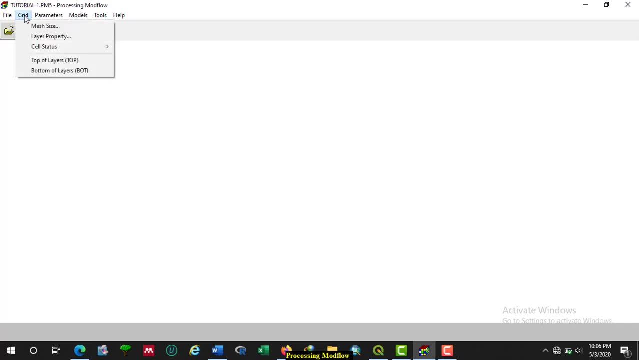 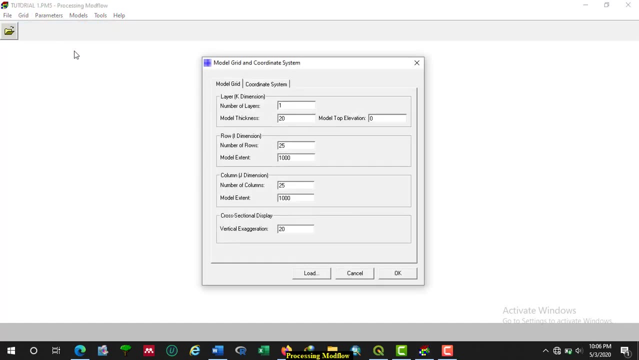 model. the first step is: what's generating the grid? to generate, agree to have quickly on. the grid turns mesh size. number of layer we have is three layer. we have three layer so we have to specify as three model thickness is what? 10 meter, which is equivalent to the. 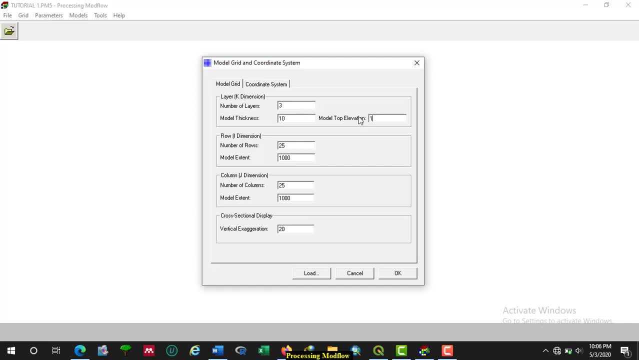 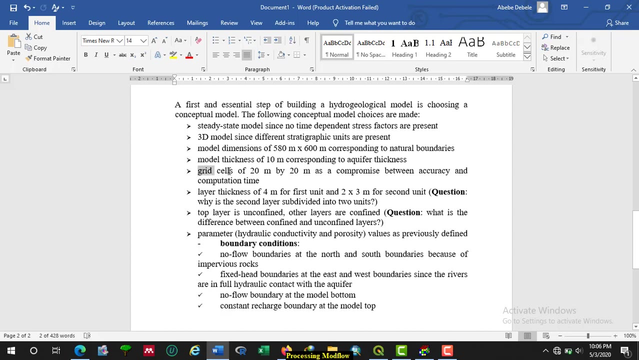 thickness of a cleaver and the model top elevation is also 10 and also we have to specify number of row and the number of column. you can look at conceptual model and the grid size is 20 meter by 20 meter and the extent of our model is. 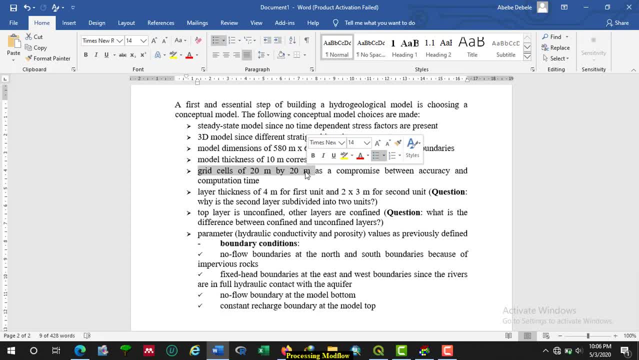 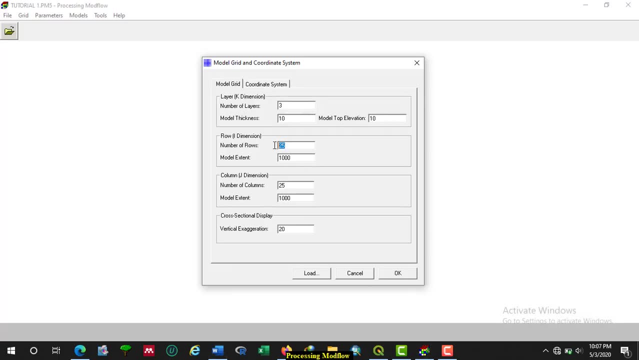 600 by 580. so if we divide 600 by 20 you can get 30. say so 30 column by 30 row. so we have to specify row as 30 and also 30. model extends 600. model extends 600. actually model extends of row is 580. 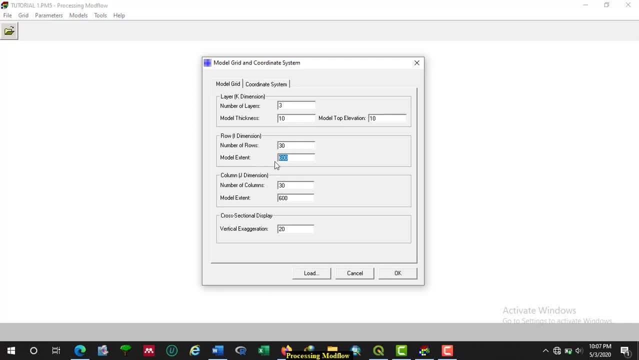 for simplification is better to make it 600. and also we have vertical exaggeration. we have to specify vertical exaggeration and when we increase the value with vertical exaggeration then the results of the model, the thickness of the vertical thickness of the model- will increase and its canvas increase the 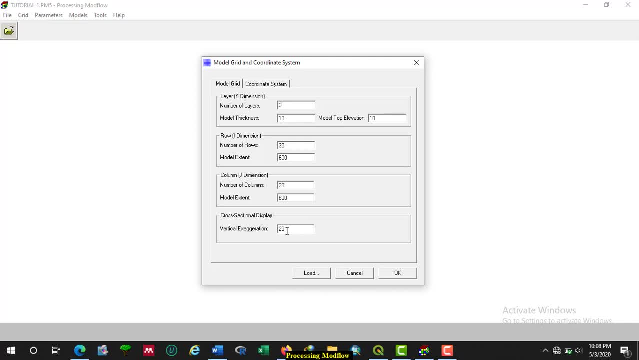 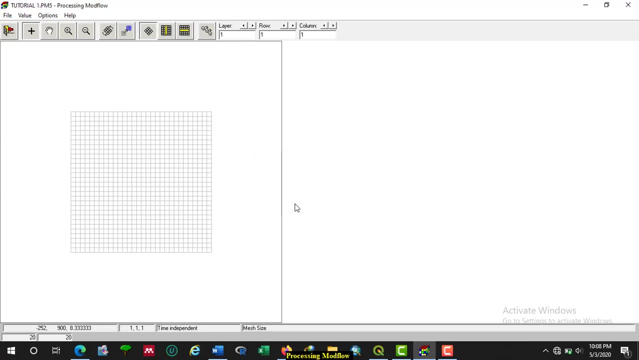 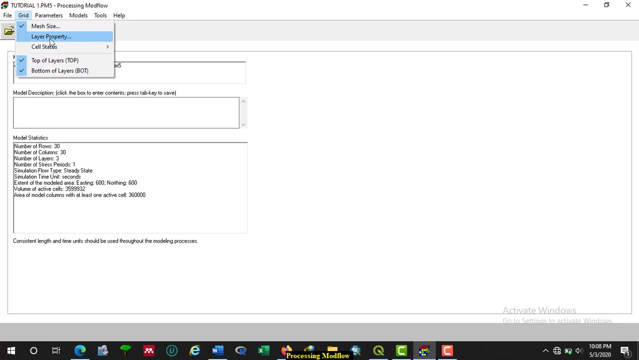 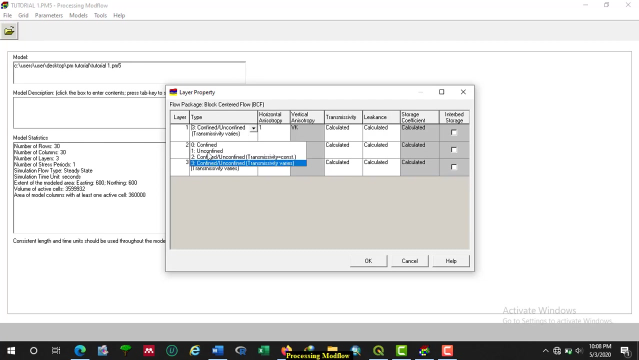 clarity of our result. for the time being, it's better to use the default value of 20 then. ok, then leave it either. and yes, the next step is what have to specify their property later property, but the first, the first occupant- i'm going find the keeper- and the second, darci cap cute. 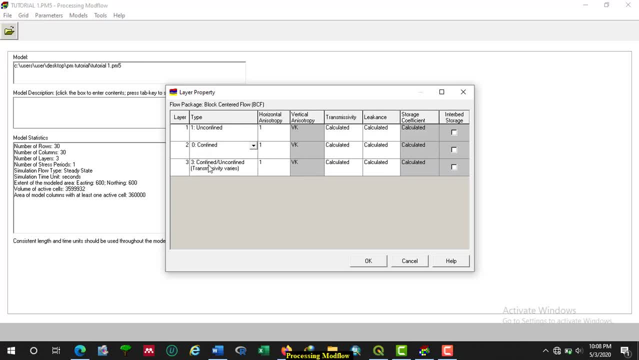 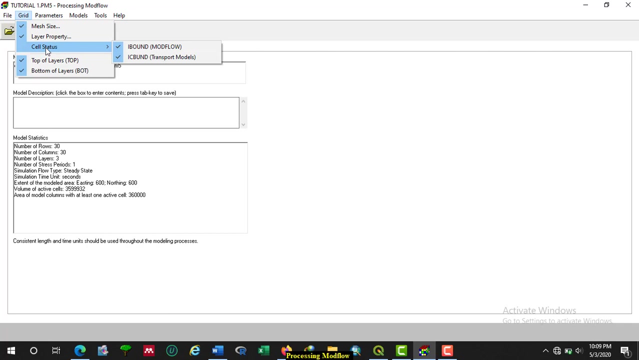 matter. second layer: arent head and they said Larry's times possible find gap layer. so we have to specify like this: then: okay, we specify the first layer as unconfined aquifer, because the problems, formulation and conceptual model also say that it is unconfined aquifer. okay, next step, we have to assign sale status. 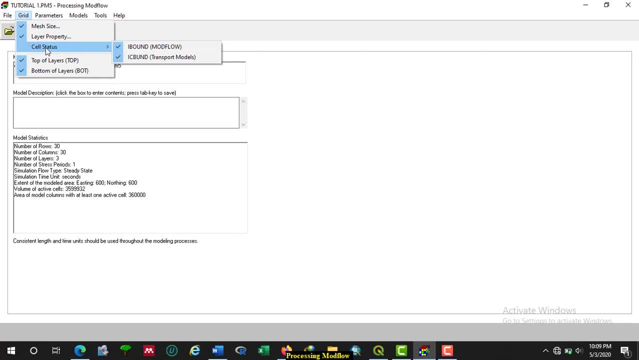 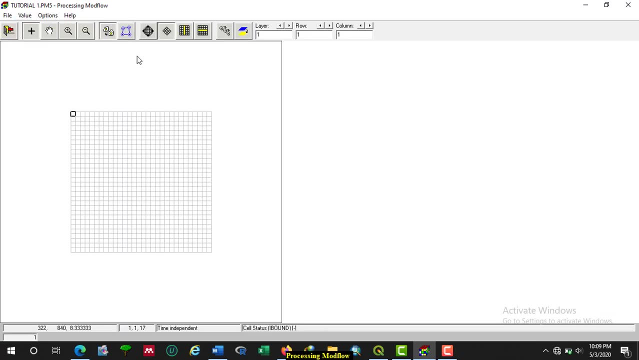 for each say to specify sales status. we have to click on create a sales status upon then, here you have to specify sales status of each say. here we you have to know how we specify sales status. when we see sales status is one, that means the sales status. 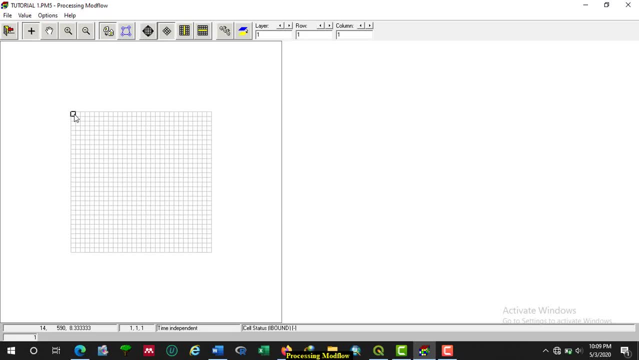 when we say this minus one, that means the sale having constant hit. when we specify as zero that sale is what in active, there is no flow. okay, in our case we have constant hit, boundary at west boundary and east boundary, so those sale should be what sale, should be what constant he and their value should be minus one, a right. 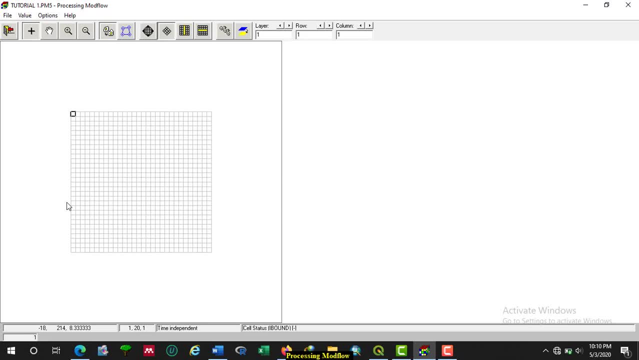 you can see this. fatning that means all sale should be minus one and all other cell should be what active. so then we click on its itself. you can see this value of our value should be minus one and all others a should be what activity say. so then we click on excel. you can see this value. 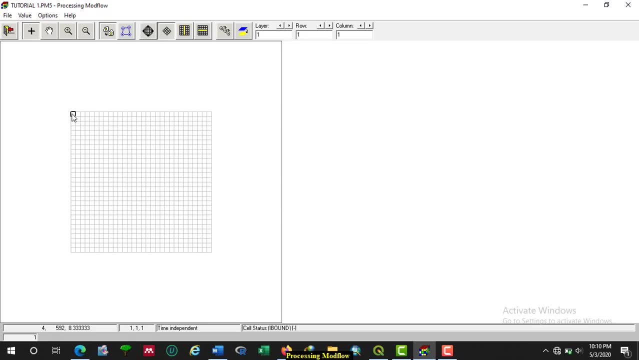 of the node boundary as constants cage. and to do that we have to click here on this cell and right click and we have to specify as minus one. then okay, so the cell status of this cell is what constant image? and we have to do the same for all cell in the waste boundary to do that. 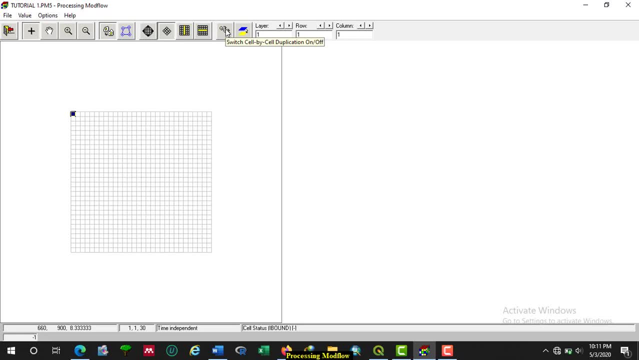 you have to click here on this button. we say: switch same by cell duplication on, then drag like this: in this case, all cell in the waste boundary are what constant image. and we have to do the same thing for all cell in the east boundary. now we assign the same status of first layer. we can look here: the first layer. 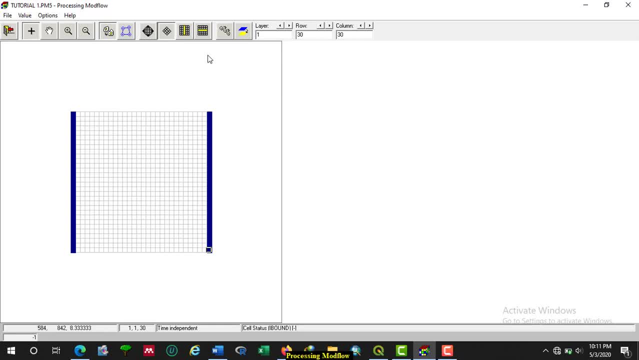 and we have to do the same thing for second length and third layer. to do that, we have to copy the status of the first layer to the second layer, the status of second layer to the third layer, the status of the same status of, uh, the first layer, sadly, and 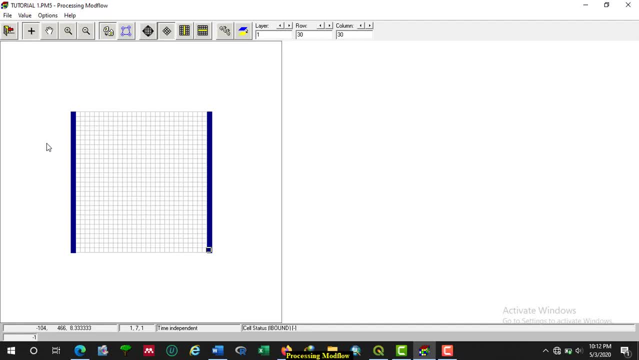 second layer the same in our case. per the problem formulation, to copy the status of the first layer to the status of the second layer we have to click on switch layer or cross section, copy all and then click this button. now the status of the first layer is copied to the status of. 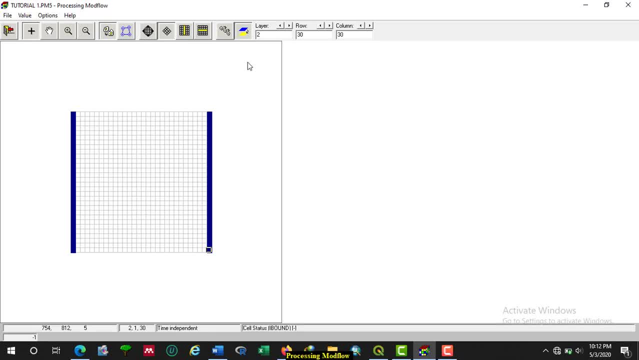 the second layer and we have to do the same for the set layer. click this one now we already specify or we already assign the status of what all layer in the first layer, in the second layer and such there. so we have to save our input. to do that, we have to click here on. leave it there. then save change to sale status. yes, 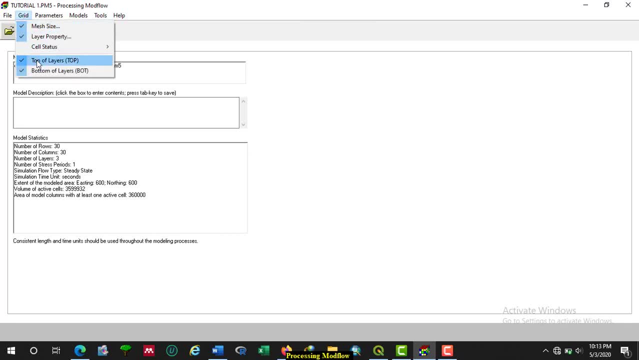 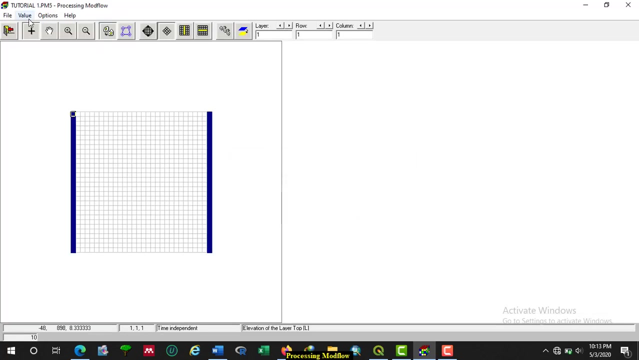 then the next: we have to specify the top layer elevation and the bottom layer elevation. to specify top, top of layer elevation we have to click on top of layers. and then the next: we have to specify the top layer elevation and the bottom layer elevation to click no. then we have to specify the top elevation by clicking value, then reset matrix 10 actually. 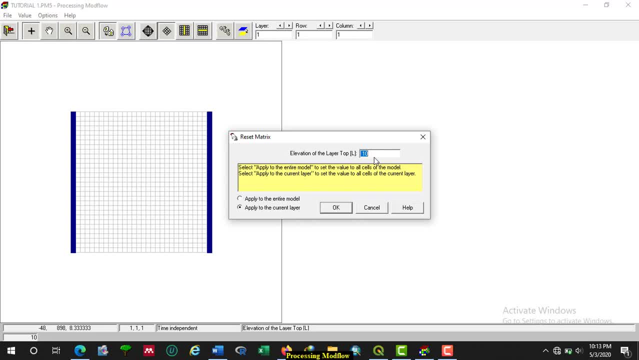 the thickness of the keyfair is 10 and also the top elevation of the first layer is 10, and we have to do the same thing for second layer. what is the top elevation of second layer? top elevation of second layer is equal to six, so we have to specify that. 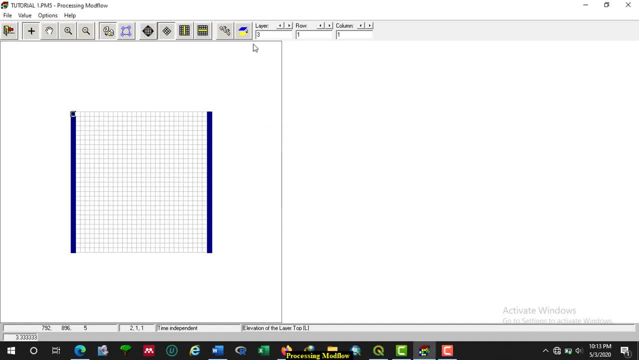 this, okay. what is the top elevation of third layer? the top elevation of third layer is three meters, because the pumping well is stand or what. the third layer and the thickness of a certain layer is what? three meters. so it is. top elevation should be three meters. okay then. 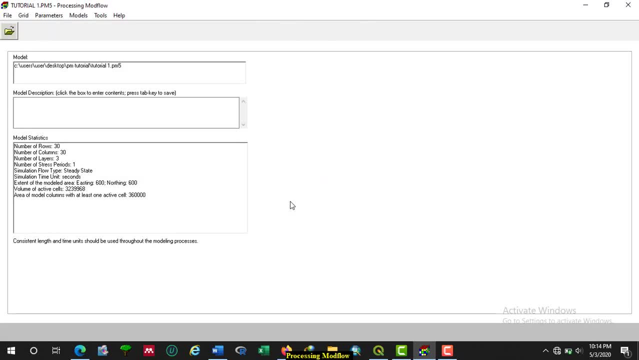 leave it here? then yes, and it is the same. we have to specify also the lp bottom elevation of each layer. to specify the bottom elevation, obviously you have to click on grid, then bottom layer, and this window is pop-up. the cover top elevation has been specified. that is what we have been. 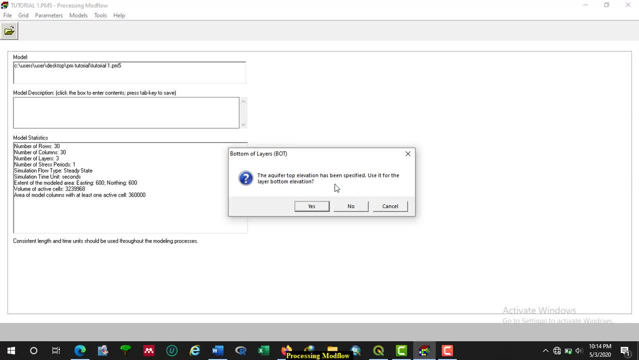 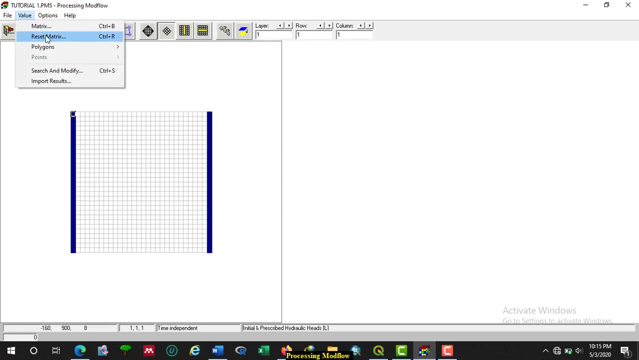 done and the software by itself can use that value to assign the layer bottom elevation. so we can say yes and leave it data and accept. then the next procedure is what specify the initial and prescribed hydrolocate? to specify initial prescribed metric, to click value, receive matrix, reset matrix and while specifying initial and prescribed hydrolocate for the model, it is better. 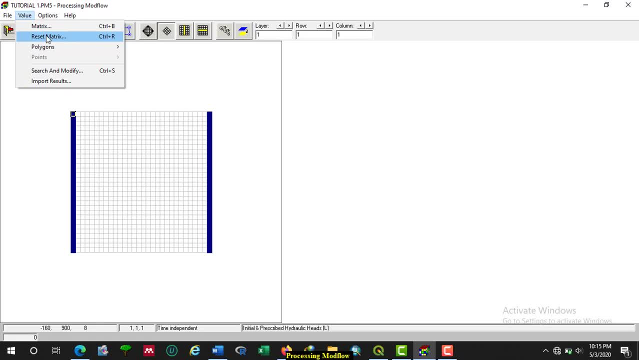 to assign initial and prescribed hydrolocate equal to the thickness of the model. so let us do that. but the thickness of that is equal to 10, so okay. however, we know that the initial hydrolocate of west boundary is nine and initial hydrolocate of is the boundary is eight, so we have to specify. 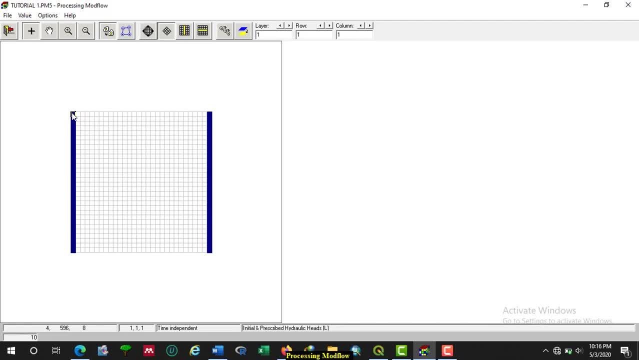 that one. to specify it we have to click here on reset right click, then specify nine and okay and we have to drag this value to all cell in the west boundary to drag. we have to click on this button then drag this value and we have to specify the initial prescribed head of what: the east boundary, because it is. 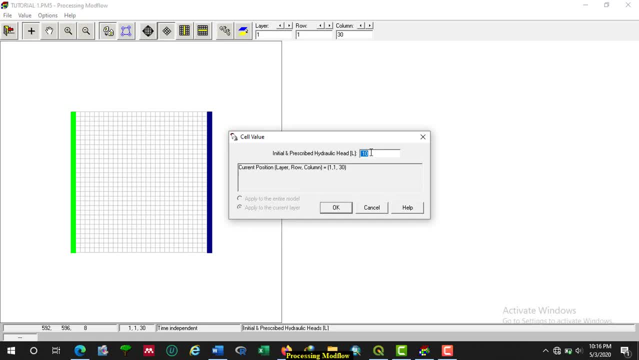 now we have a constant head of eight, so we have to specify this one then. okay, then we have to copy this value to all cell or we have to duplicate it to also in the east boundary. okay, we define or specify initial and prescribed hydrolocate of what first layer? 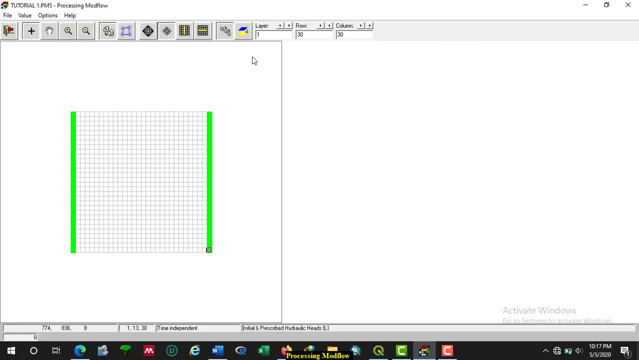 to do also for the second layer and third layer. in our case initial prescribed hydrolocate of first layer is equal to initial hydrolocate head of second layer, equal to initial hydrolocate of a third layer per problem formulation. so we have to copy the value given for the first layer to 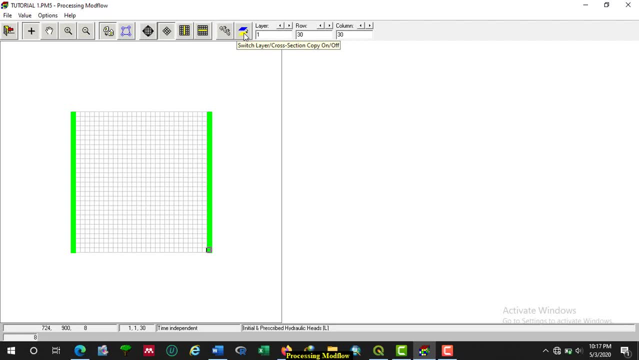 the second insert. to do that we have to click here on switch layer or cross section copy on, then click this button and this button. okay, now initial and prescribed hydrolocate of first layer is copied to the second and the third and initial- i call hydraulic. initial and prescribed hydrolocate is already specified for layer, so we have to click this, leave it there. 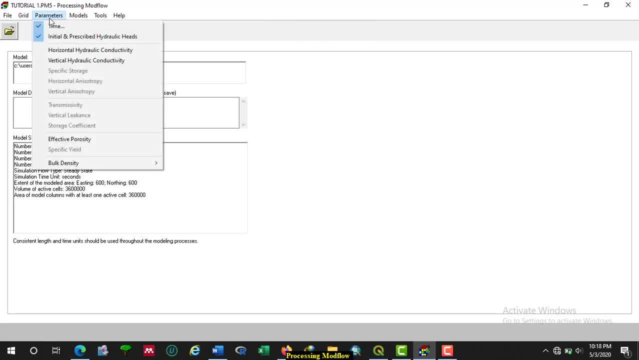 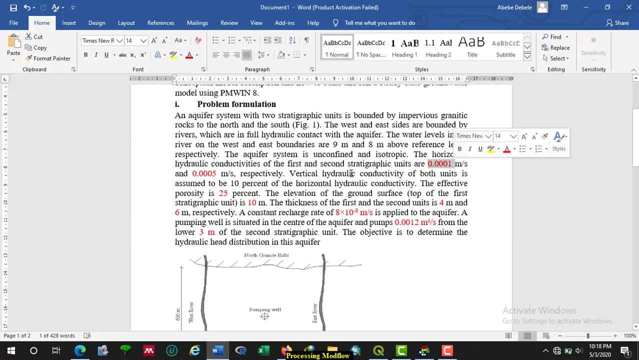 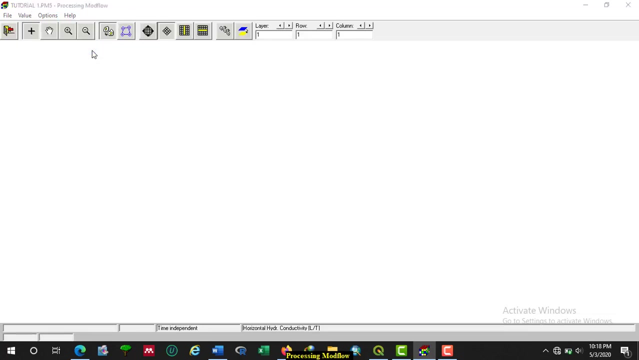 then yes. the next procedure is: what is specifying horizontal hydroconductivity? we now horizontal hydroconductivity of first layer, horizontal connectivity of first layer- is this value? and horizontal conductivity of second layer and sub layer- is this value it is specified to specify horizontal connectivity. you have to click here on horizontal conductivity. 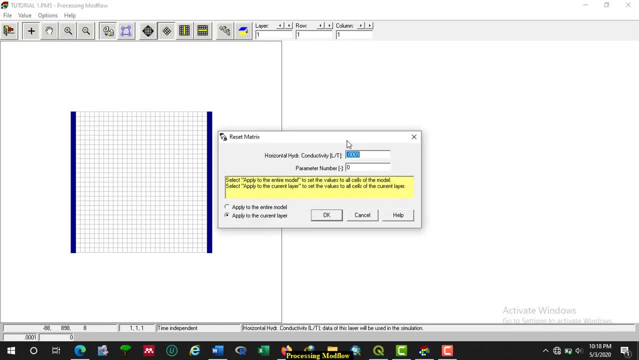 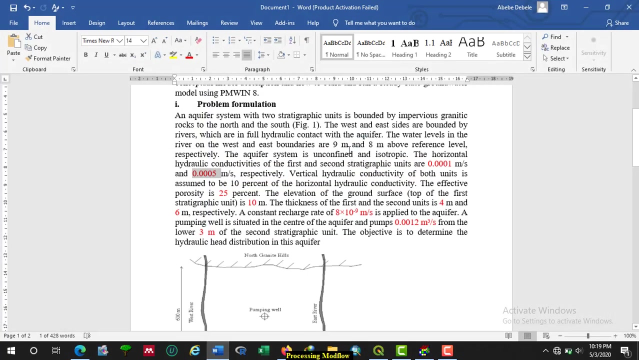 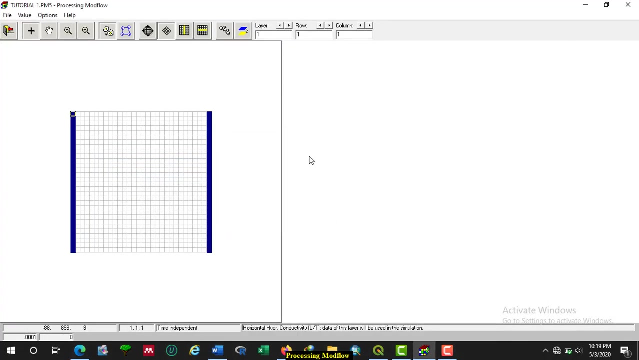 and value receipt matrix. by default, horizontal hydroconductivity of first layer is equal to 0.001, and this value is the same to the value here given in our location, so we have to accept this one. okay, we have to do the same thing for second layer and we have to click on value. 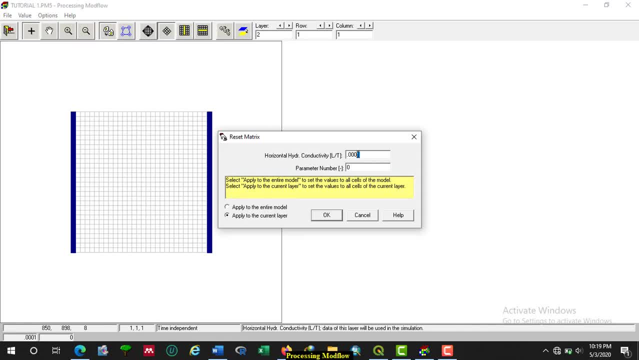 receipt matrix. but in this case, horizontal conductivity of second layer is not 0.001, it is 0.005. so we have to specify like that and okay, and we have to do the same thing for sat layer. horizontal hydroconductivity of certain layer is equal to 0.005. 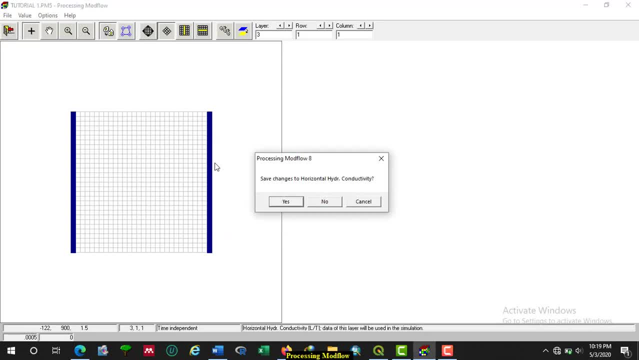 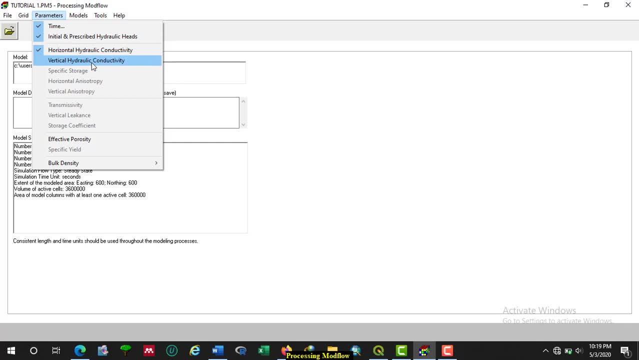 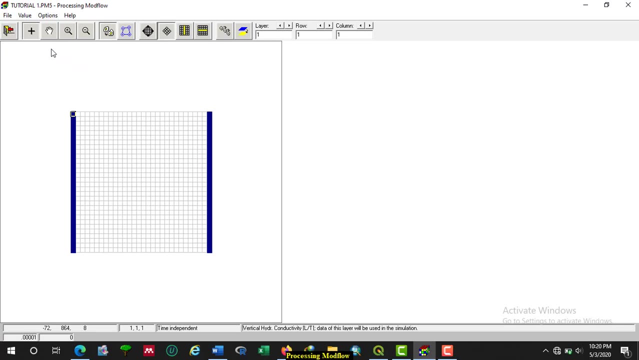 then okay, leave it there. yes, we have this space by also vertical hydroconductivity. specify vertical hydroconductivity, click vertical hydroconductivity, then value reset. matrix: vertical hydroconductivity is 10 percent of horizontal undo conductivity, so this value is equal to 10 percent to horizontal hydropon activity. 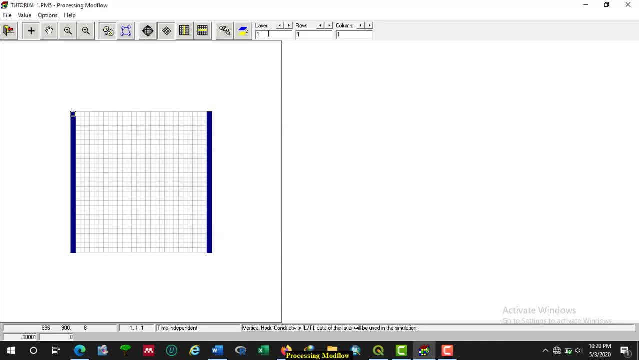 so accept and let's specify for second layer: click here, then value reset matrix. let's change this value to zero point, zero point, zero, zero, zero, zero, five. then okay, for sub layer also new value reset matrix: zero point, zero, zero, zero, five meter per second. okay, then let me do that. save. change to vertical. 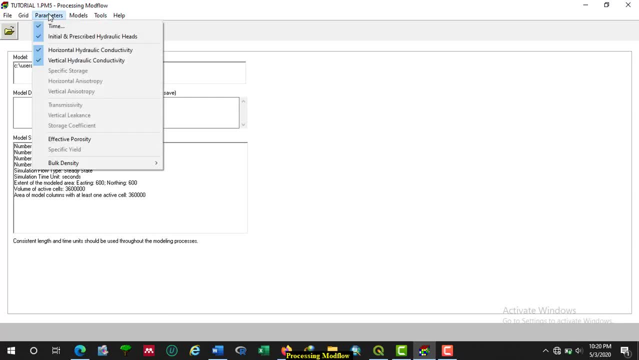 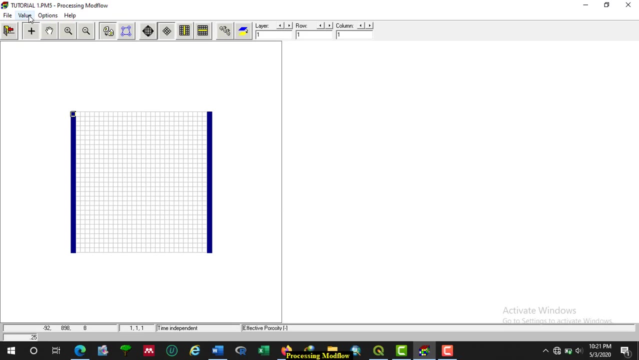 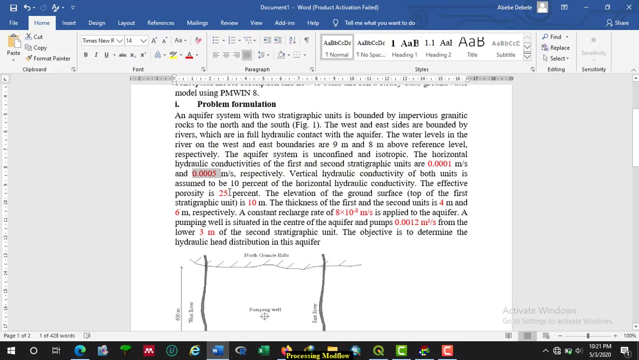 hydropon activity. we specify initial prescriber: liquid horizontal conductivity. vertical hydroconductivity was left. effective force is left, so click on effective porosity. specify. specify effective porosity value. reset matrix. the default value of effective porosity given to the model is equal to, here, effective porosity given in the problem. 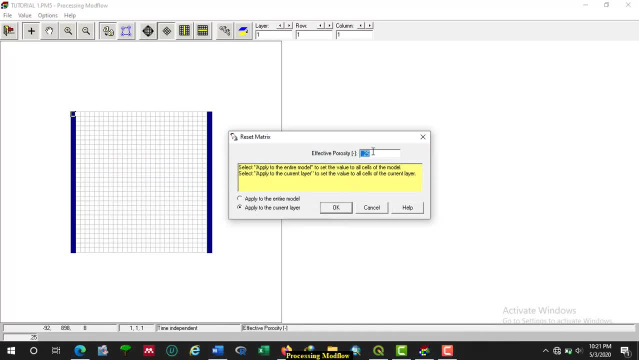 formulation. so we have to affect, we have to accept this default value. accept and let us check for second layer. second effect, hydroconductive effective porosity for second layer is also zero point zero five. effective porosity of third layer is also zero point two five. so we have to accept that this is, then leave it either. then yes. 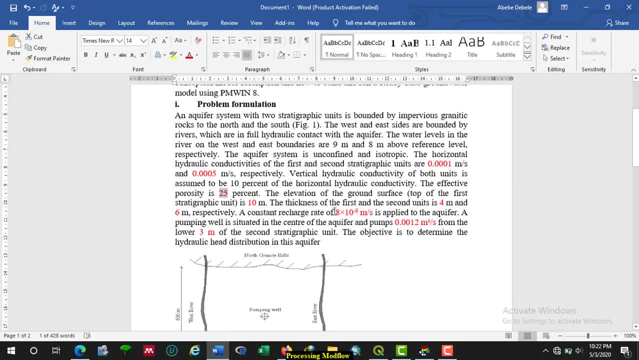 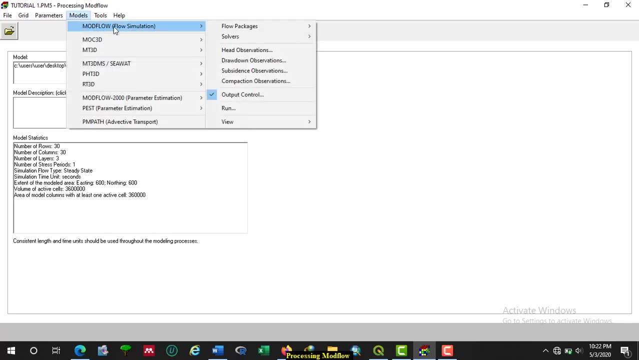 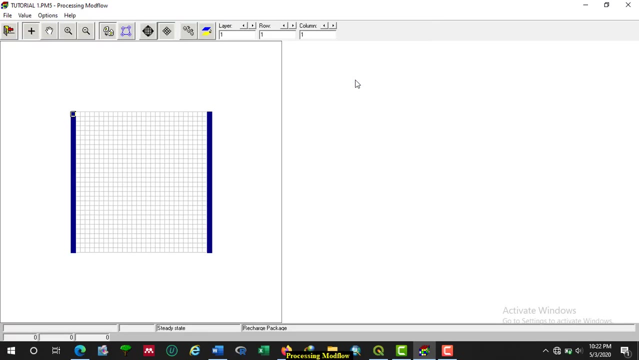 another parameter we have is what recharge. so we have to what specify this one recharge? to specify this recharge, you have to click here on model, then flow simulation, then flow package, then recharge and recharge is what? to the first layer, only to the first layer. this precipitation, and the precipitation is 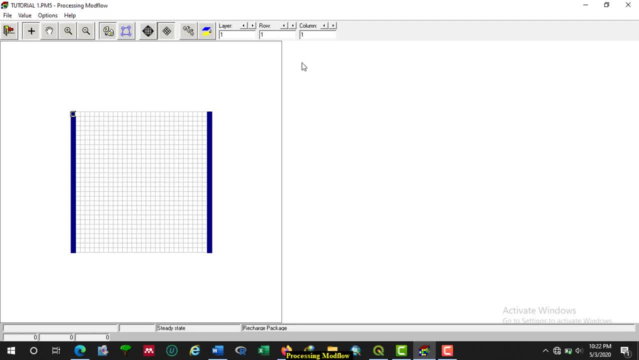 from the top and this to the first layer. so we have to specify that recharge value to the first layer. here you can look at the layer number. this first layer value reset matrix. what is the value of recharge rate? the value of recharge rate is what? 8 times 10 to the power of minus 9. so we have to write: 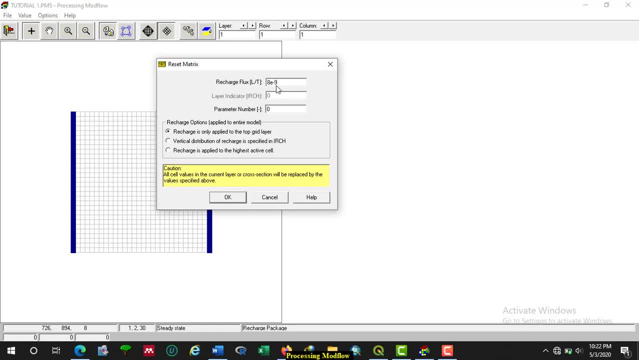 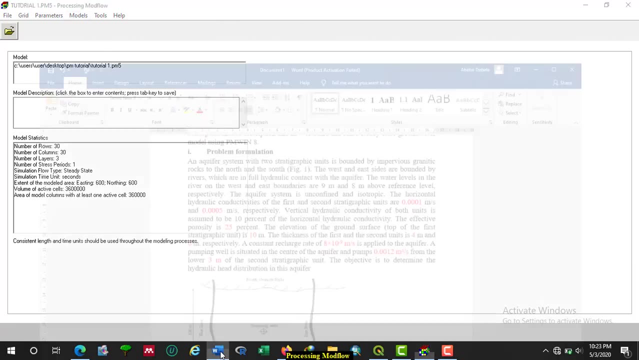 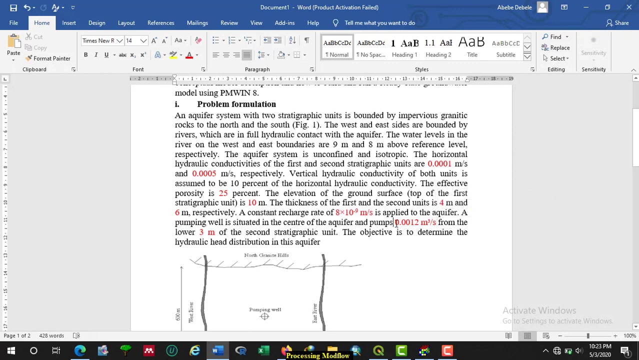 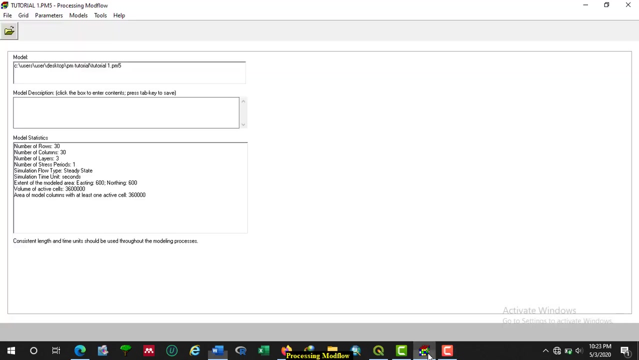 like this 8 exponent of minus 9, then okay, then leave safe chain to recharge the only lives given values, pumping rate. and this pumping well is situated at the center of a keeper from the lower three meter of a second stratigraphic unit. so we have to. 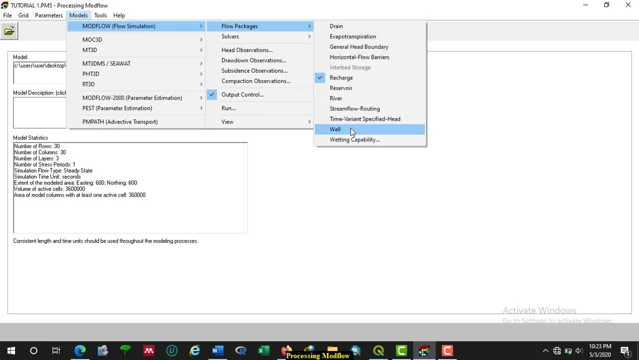 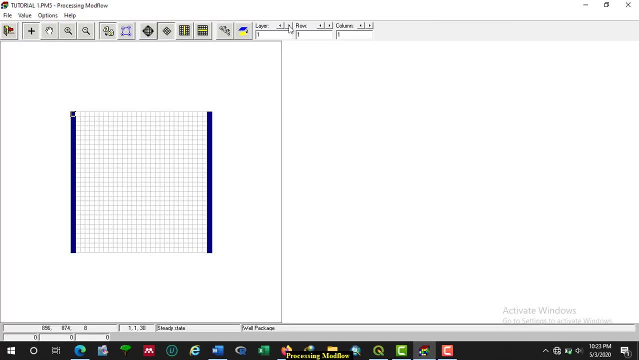 put this pumping way in the shirt there, then you have to go to certain a circular color here, and the well is what. at the center of, at the center of the key, for at the center of that keeper, that means by the dimension of the moon, dimension of our model. 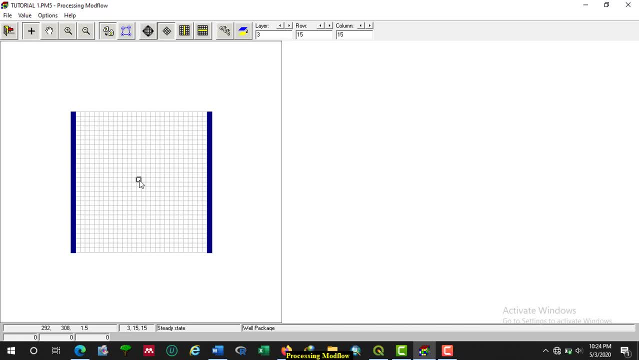 is one 30 by 30, so the center is around here, which is about 80 by 50, and we have to click this, say on this, then right click and specify the value of what: the value of pumping weight. and the value of pumping weight is equal to minus 0.0012 if this value should be negative, because 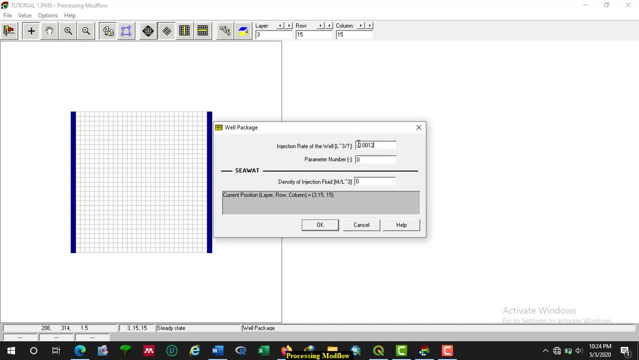 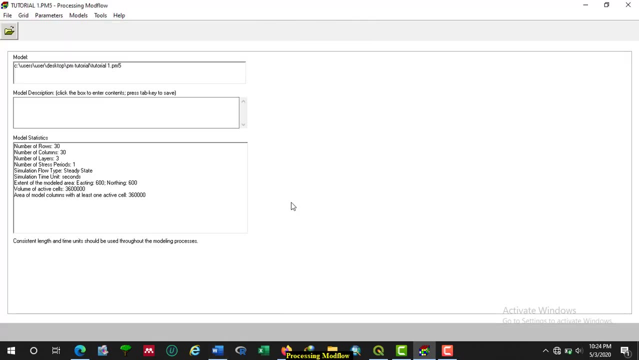 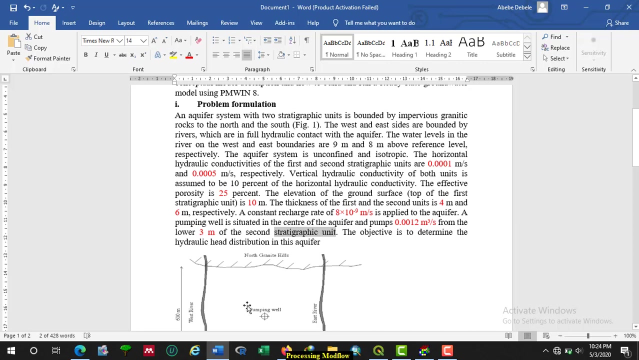 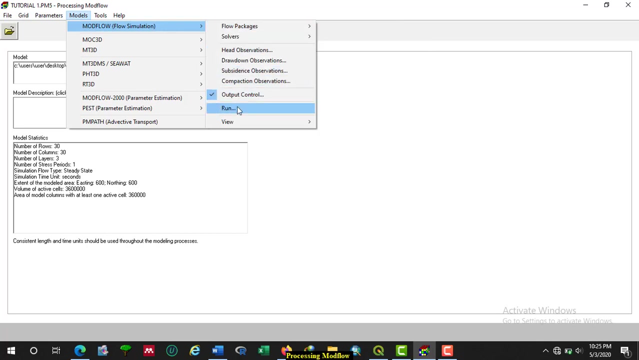 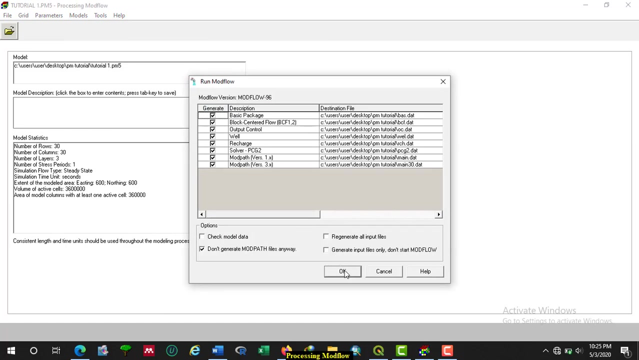 the aquifer is losing water. it is pumping, not injection. well, so the value should be negative. then, okay, leave it either. yes, we already specify all parameter given for us. so the next procedure is what? we have: to run our model. to run our model, we have to click on mode flow, then right, run the model. then this window will pop up. 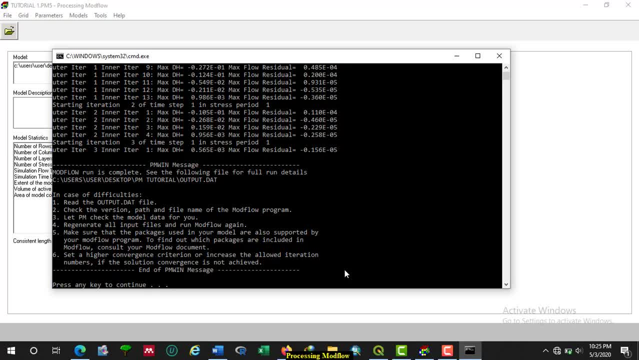 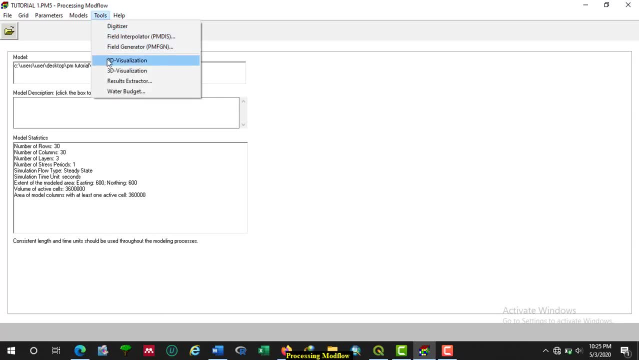 then click any k or keyboard, then black window will disappear. then we can visualize our result. to visualize our result, you can visualize 2d visualization using 2d visualization. you can visualize our result using 3d visualization, or water budget and so on. let us visualize our result using 2d visualization. 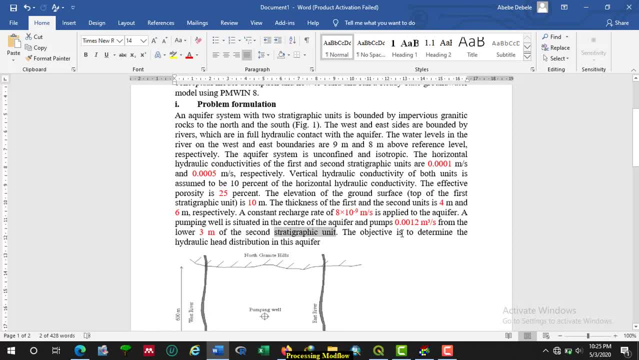 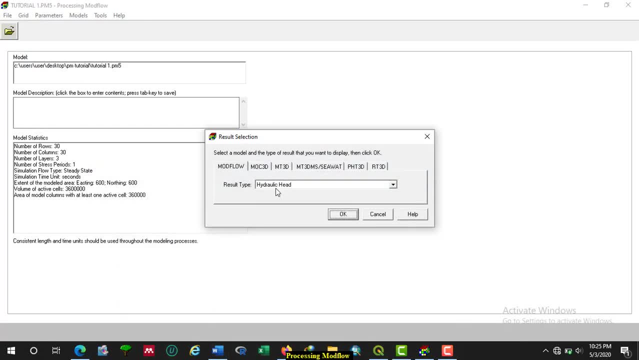 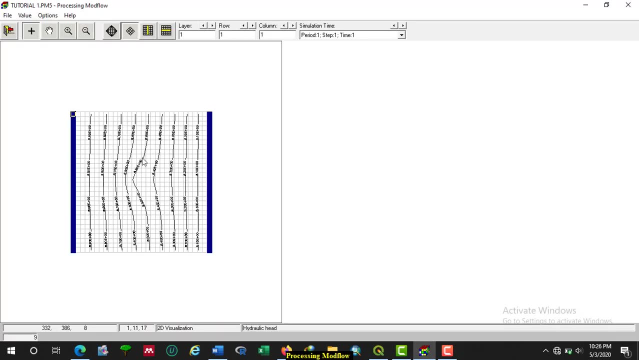 and what was our objective? the objective was to determine hydrolicate distribution in the kiffer. so we can see hydrolicate distribution in the kiffer by clicking ok, and this one is what? hydraulic head distribution in the first layer. you can click this one also. you can see hydraulic head distribution in the second layer and click. 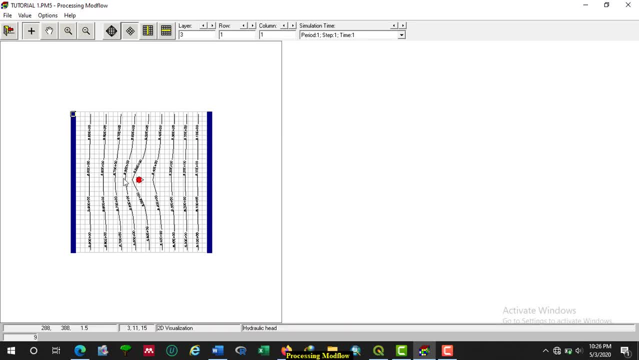 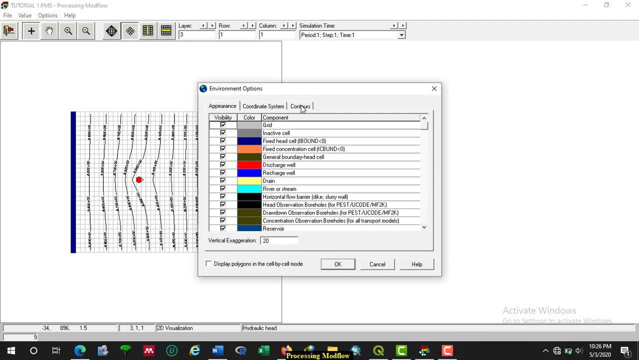 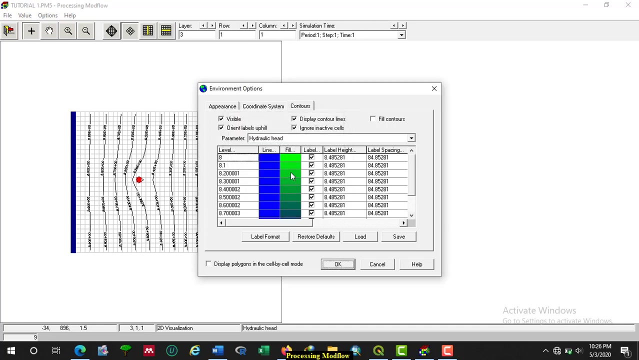 this one and see how to duplicate distribution in the second and third layer. we can decorate our hydraulic head map using option, then environment. we can change contour property. we can change the interval of our contour. we can change also the color spectrum of our contour. let us change this, this color, to red, then okay, so the minimum spectrum is what this color which is. 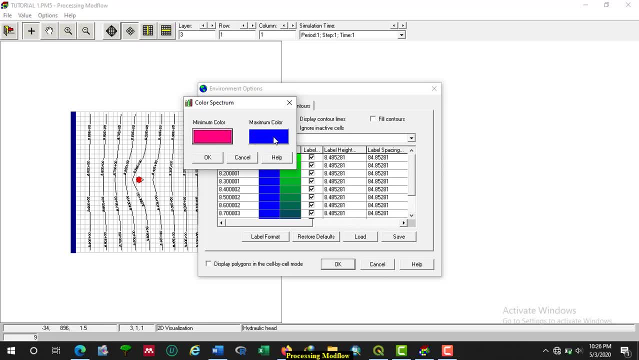 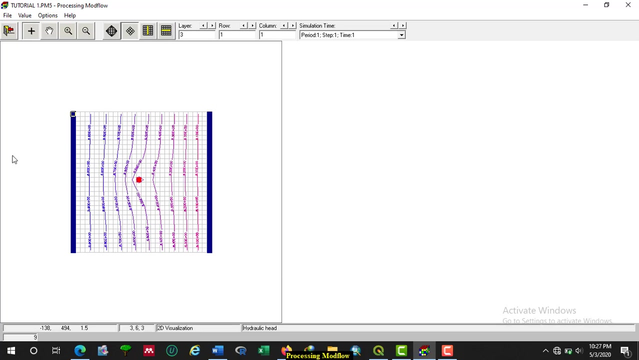 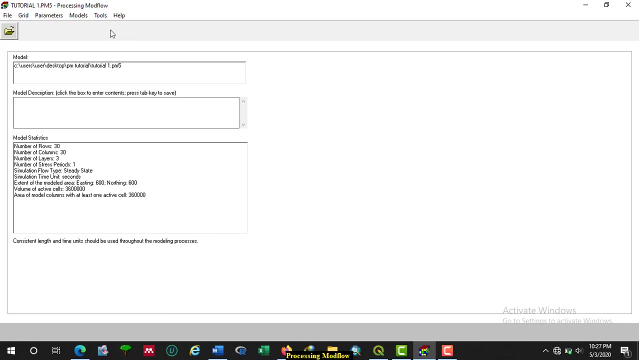 pink and the maximum one is what blue? then okay, and we can also change label format. then we can use fixed number or we can use exponential table. okay, so you can see the hydrolicate distribution map for third layer, second layer and third and first layer S rank. let me add one thing for you. let us see the water budget of our 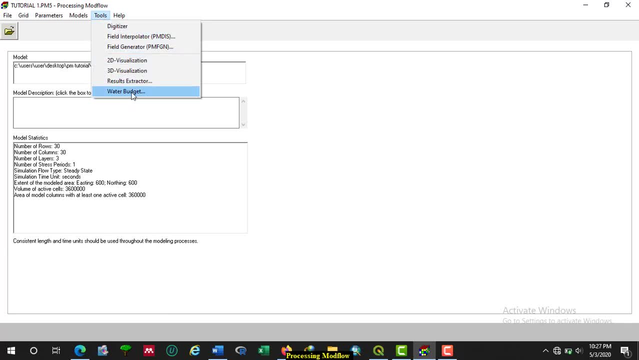 model. to see the water budget of a model, we have to click on to the water budget and straight period is 1 or steady states. a time state is 1. and let us define the subregion. we have 3 sub reason because we have three layers. Layer 1: 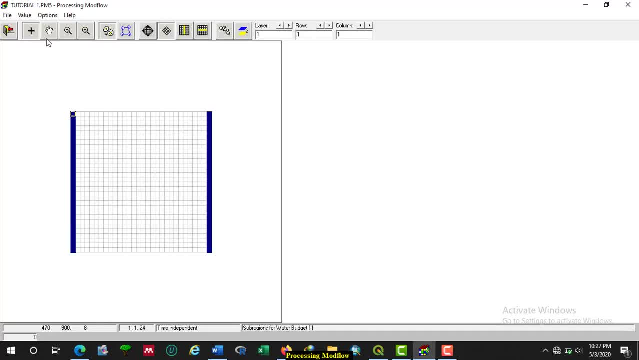 and we have three Sh. définie eighth sub region, because we and R are remove and seven belongs in state萬. excuse meического. layer 2, layer 3, define sub region. let us define layer 1 as sub region 1, so value reset matrix. 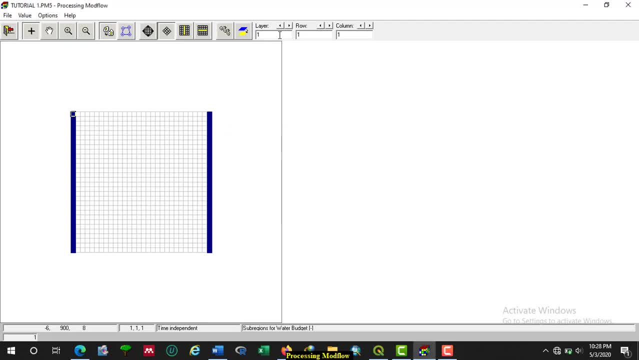 it has 1 sub region 1 for layer 2. for layer 2, let us define it as what? sub region 2, sub region 2? okay, let us define layer 3, layer 3, as sub region 3, sub region 3, then okay. 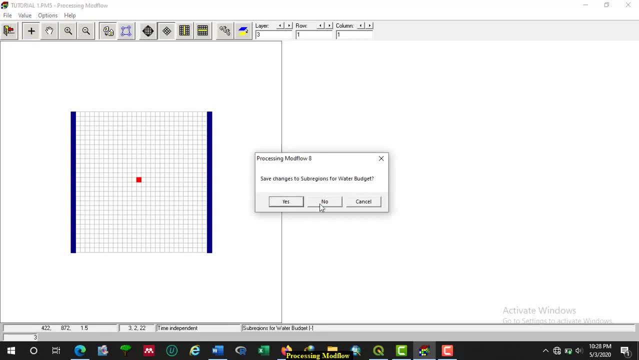 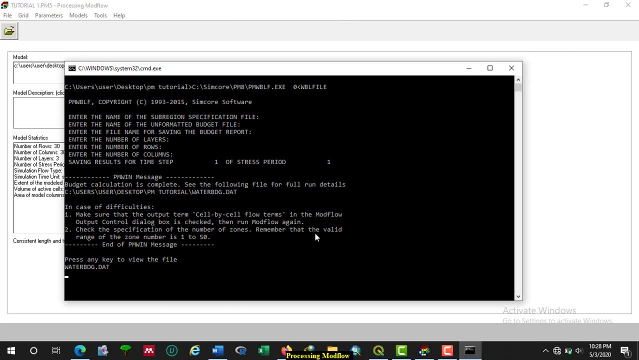 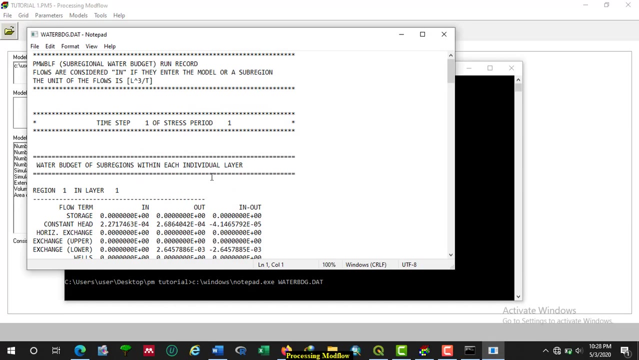 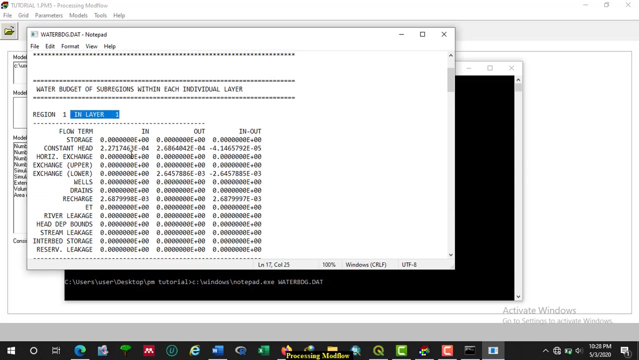 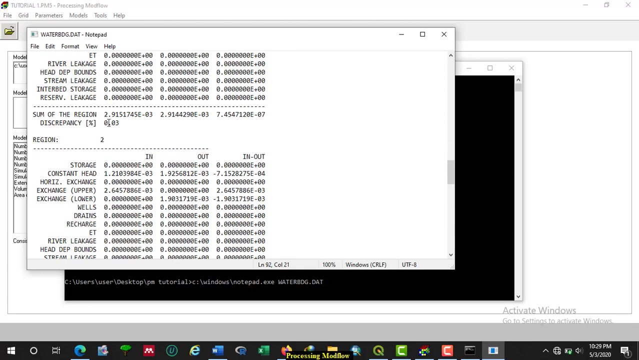 then leave it either. then yes, then okay, okay, then click any key on keyboard, then this value will pop up. this is what water budget of what? our model: water budget of layer 1. water budget of layer 2. water budget of layer 3. or you can see region 1, which is layer 1. 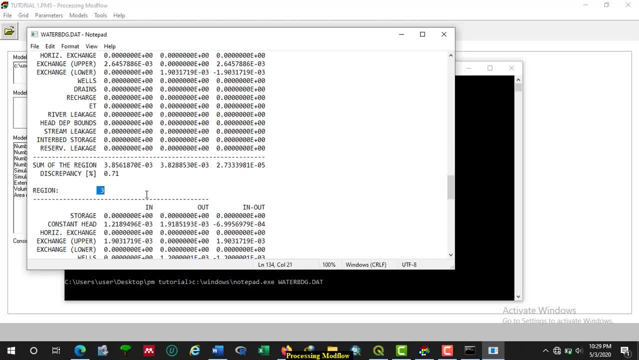 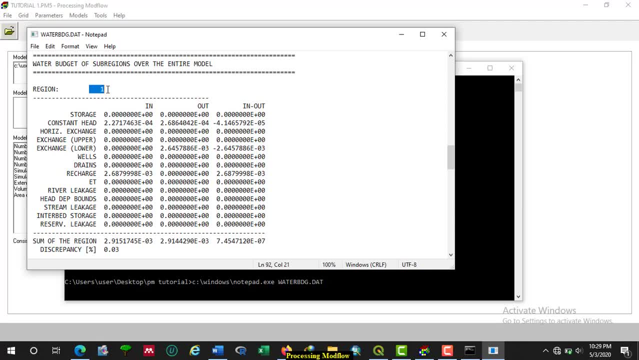 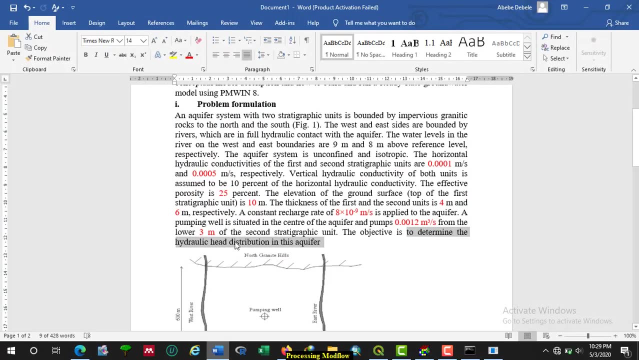 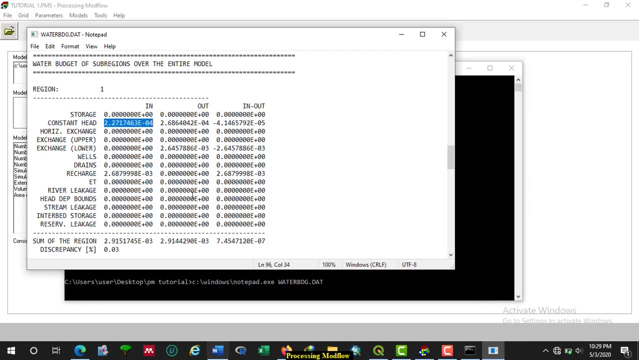 region 2, which is layer 2. region 3, which is layer 3. let us see water budget of what each layer look at: layer 1 or region 1. this amount of water is what flow from. this amount of water is flow from river to this aquifer or layer 1, and this amount of water. 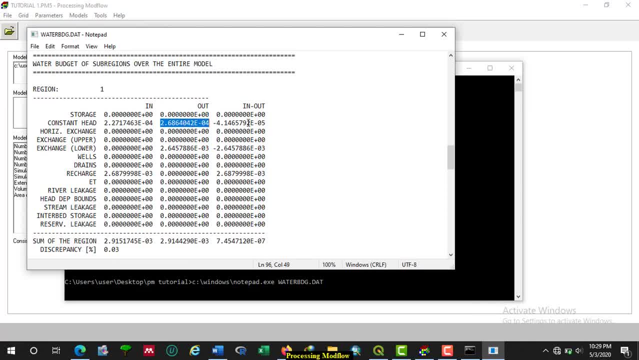 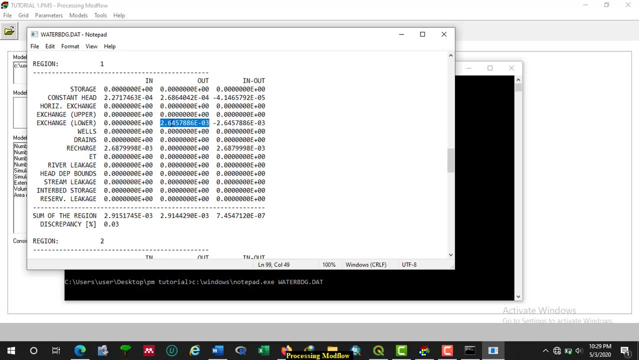 is flow out of layer 1 to the river. so in this case there is negative exchange and we have also another flow which is lower flow. that means this amount of water is what flow from aquifer one, two, or from layer one to layer two. so still there. one is what losing weather.